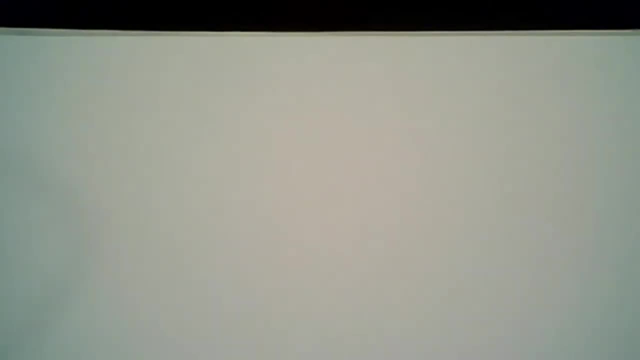 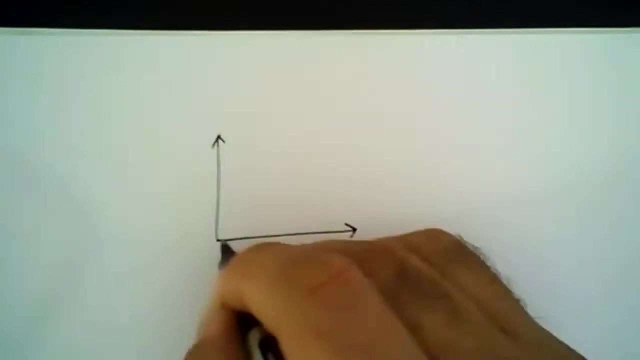 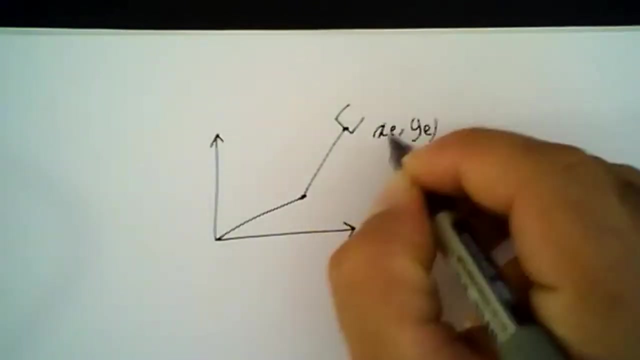 Hello guys, in this lecture we're going to continue our work and today we're going to cover differential kinematics. As we all know, if we were to calculate the inverse kinematics of a, let's say, a two-degree freedom robot, in this case we would have the coordinate. 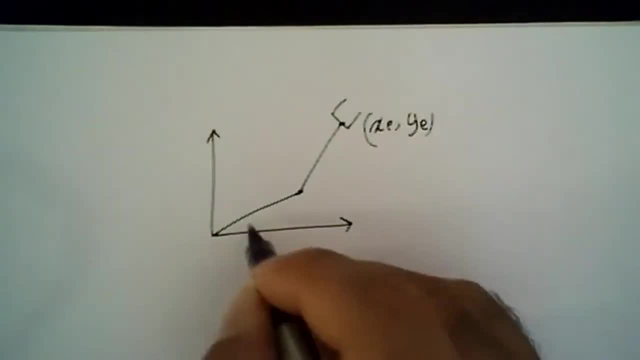 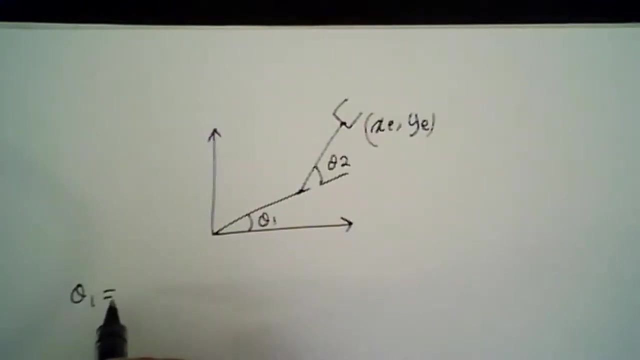 of the ended factor, and the goal of the inverse kinematics is to calculate theta1 and theta2.. And in this example that we had last time, we used inverse kinematics and what we did is we solved theta1 as inverse kinematics, basically inverse tangent of y e over x e. 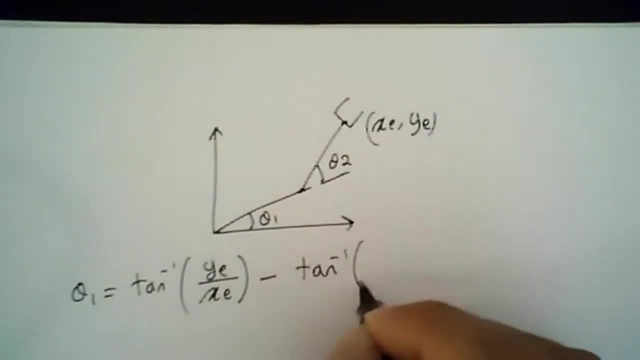 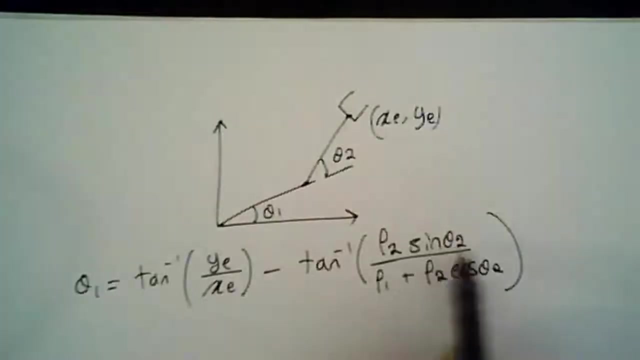 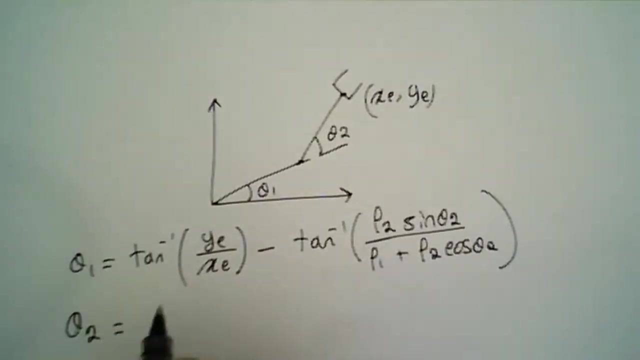 minus inverse tangent, minus y e, And we had solved theta2 based on the geometry of this and we said that theta2 was equal to inverse cosine of x e squared over y e. So theta2, plus y e squared minus l1 squared minus l2 squared. 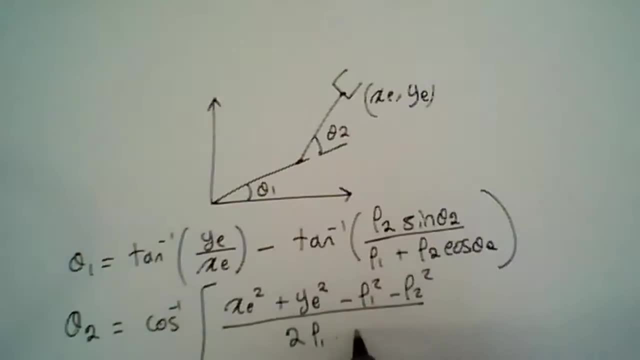 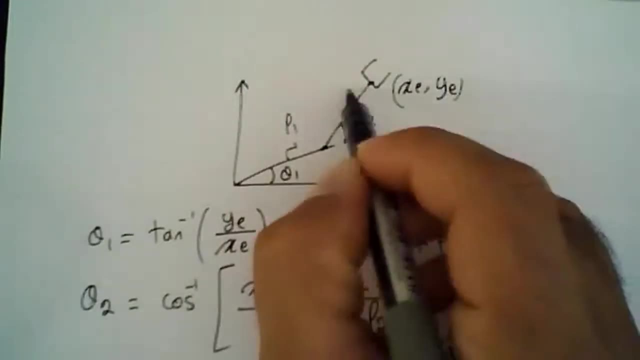 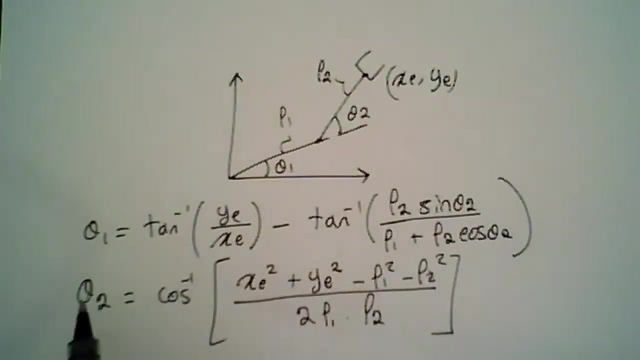 And this whole thing was divided by 2, l1 multiplied by l2.. And we know that the link length here is l1 and the link length here is l2.. So once you have x, e and y, e, you can calculate theta2.. 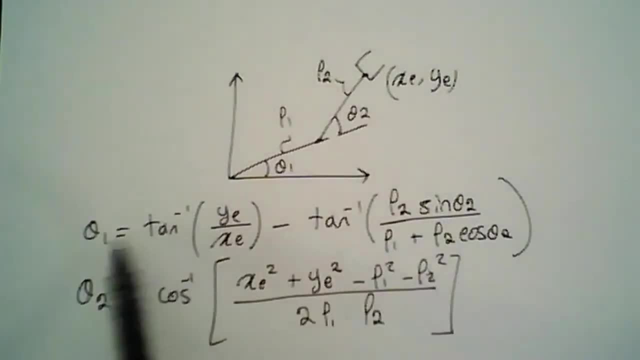 And after you calculate theta2, you can calculate theta2.. So here you have x, e and y. e replace it in this equation and you can calculate that one primarily based on xe and yu. so sometimes the geometry of the robot will actually make it very difficult to obtain. 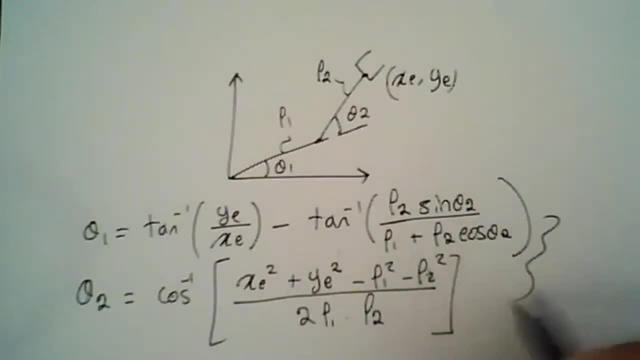 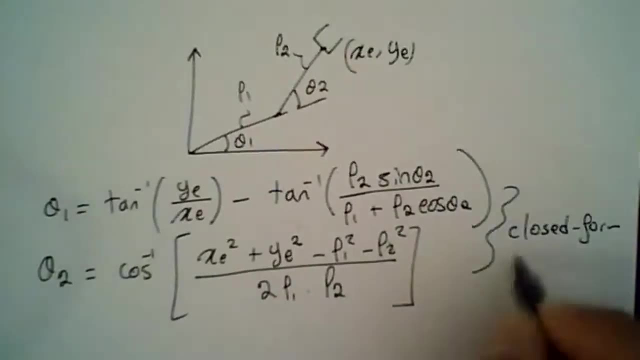 this closed form solution, right? so this is referred to as a closed form solution, and this is not always feasible. so instead, what we can do is we can actually apply a differential kinematics and we are going to be able to find that the one and the two are based. 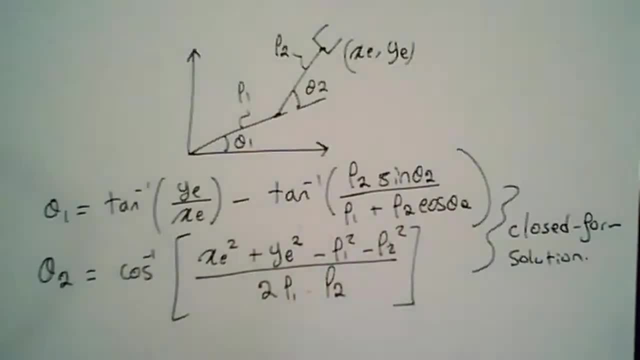 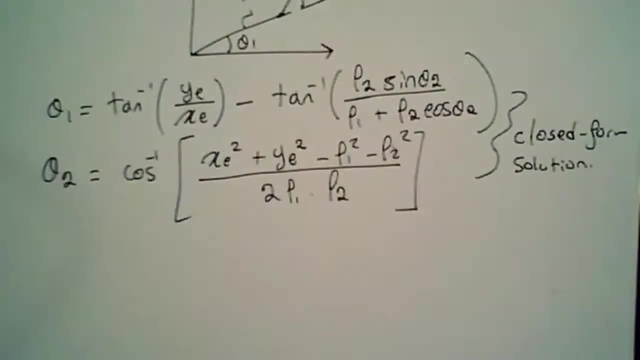 on xe and ye without actually having to, you know, figure out all the geometry, and the approach is actually pretty straightforward. so what we'll do is we will use forward kinematics, we differentiate forward kinematics and we can obtain a relationship between the x and the data right. so let's see how. 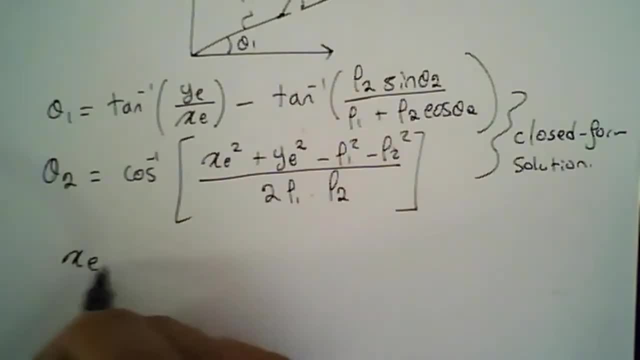 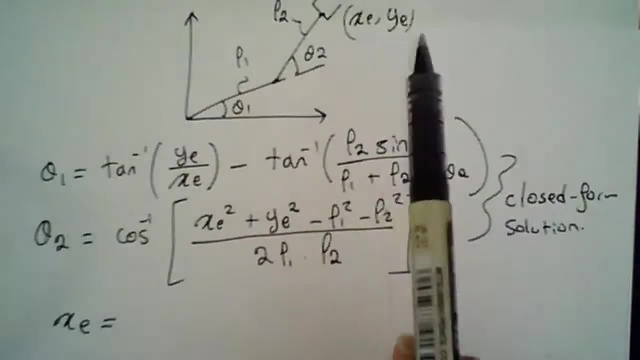 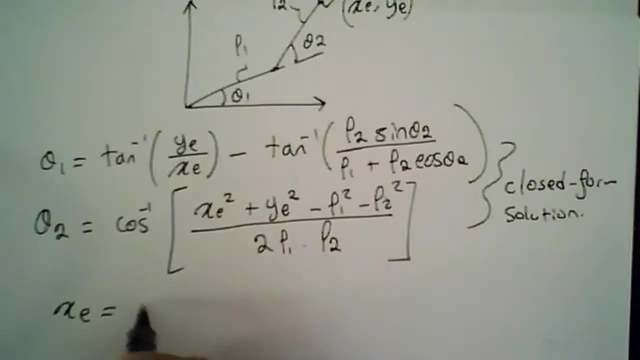 that is actually implemented. so what i'll do is i can begin by writing xe, right? so the forward kinematics of this robot is going to be: i need to be able to represent xe and ye in terms of theta1 and theta2, right? so what is x? in this case, it's going to be l1 cosine, theta1. 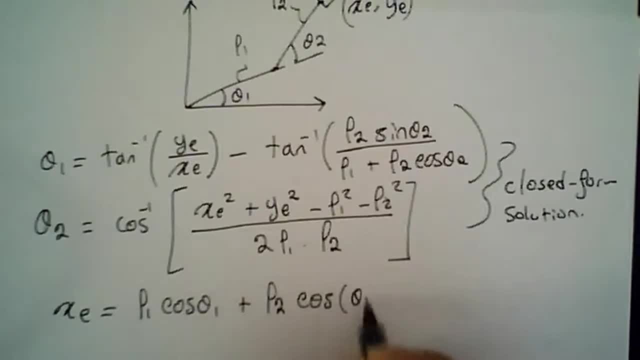 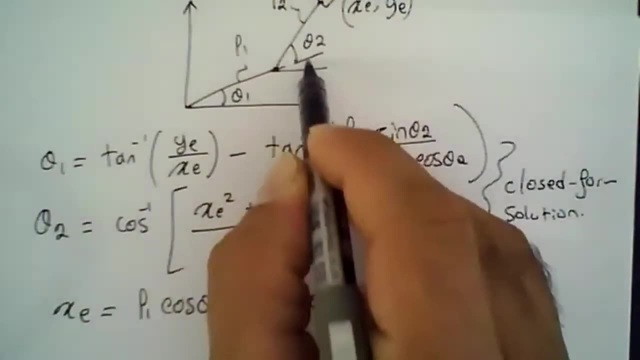 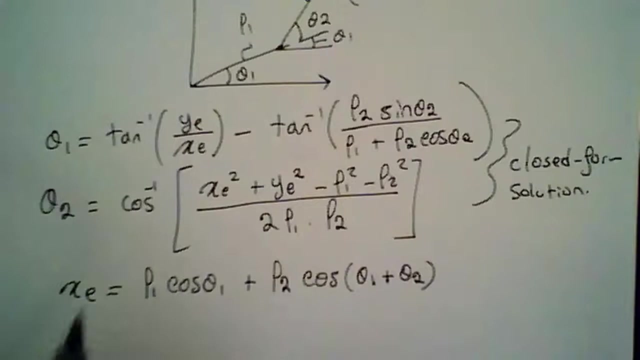 plus l2, cosine theta1 plus theta2, because we know that theta2 is only relative to theta1. so here we have theta1. so if i was basically projecting that obviously it has to be cosine of theta1 plus theta2. and how about ye? ye is going to be equal to l1 sine theta1 plus l2 sine of theta1 plus theta2. 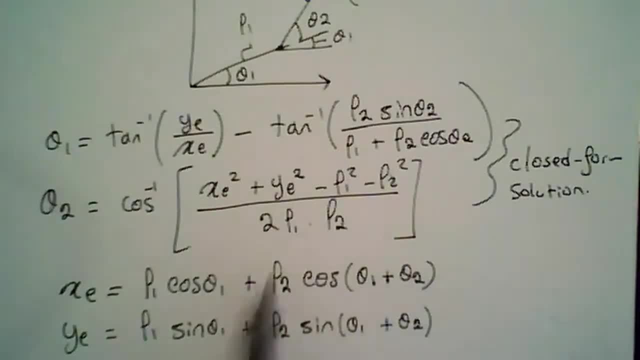 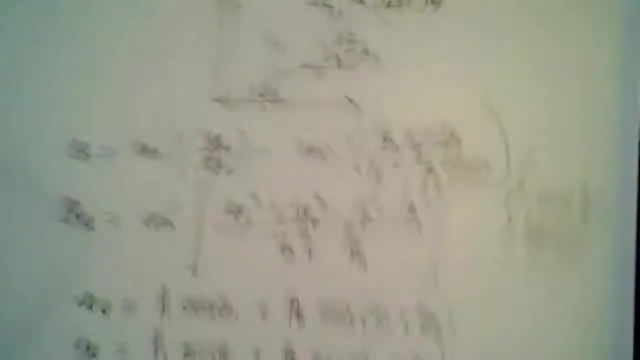 all right. so obviously, the goal is to actually solve that one and, as you can see, you know, this is a highly nonlinear equation and it's very hard to basically pull that down and then from this to solve it. so what we can do actually, uh, we can differentiate this guy and by differentiating, 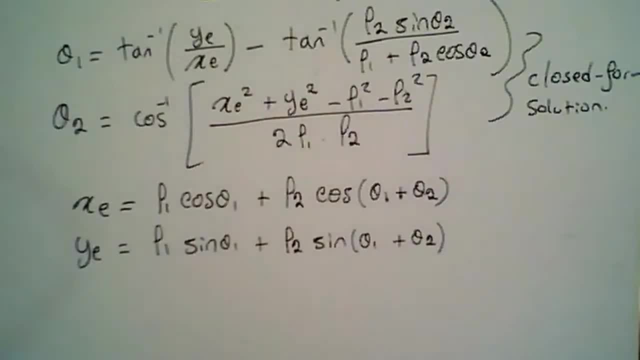 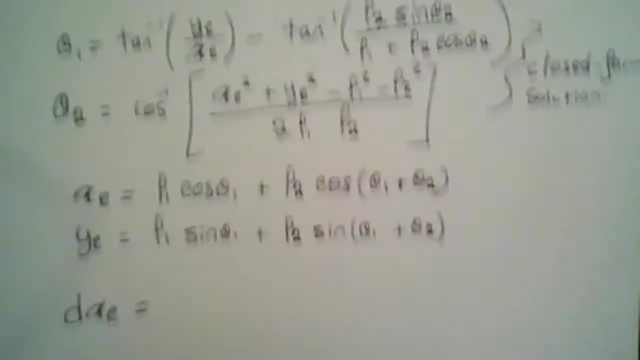 that we can actually obtain a relationship between uh 1 and 2.. so what is uh? so xe is a function of theta one and theta two, so it's a multi-variable function and if i were to differentiate the xe, i'm gonna have to do this right, i'm gonna have to do it here. actually. partial derivative of. 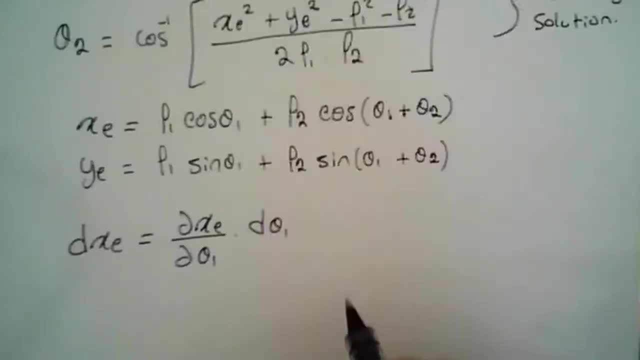 to delta one. multiply the square by delta one. right Plus partial derivative of Xe with respect to delta two, multiplied by delta two. All right, and I'm gonna do the same thing on Ye. So what is Dye? Dye is gonna be equal to, again, partial derivative of Dye. 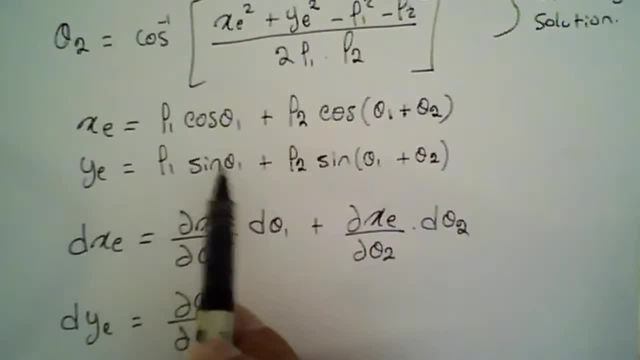 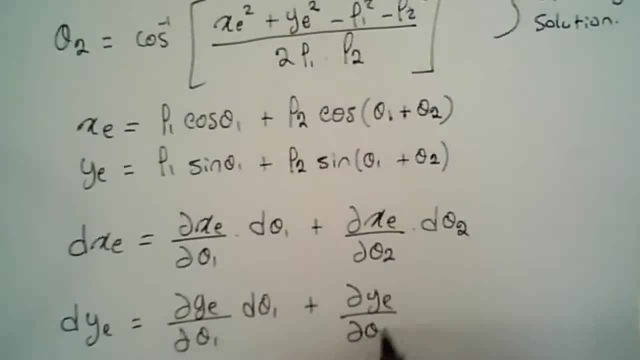 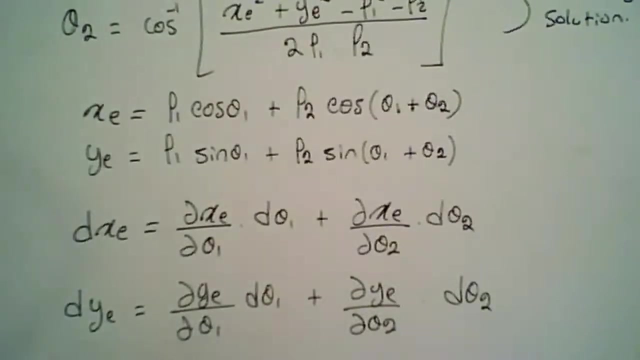 with respect to delta one, because Ye is also a multivariable function of delta one and delta two. So delta one plus Dye with delta two multiplied by delta two. So if you actually look close here you can see that we can basically put this: 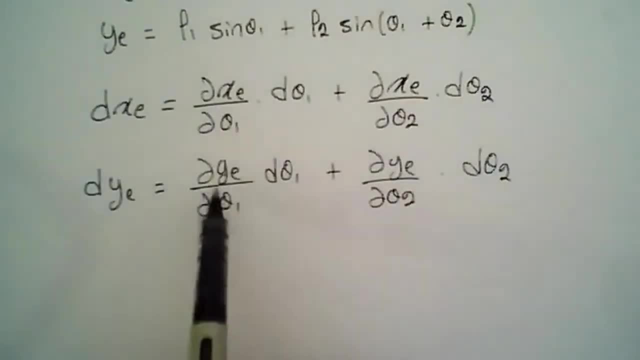 as a matrix operation right, Because you have you know, delta one basically is applying, is applied here and here, and delta two is applied here and here. I can actually rewrite that as a matrix format, Dye, Dye right. 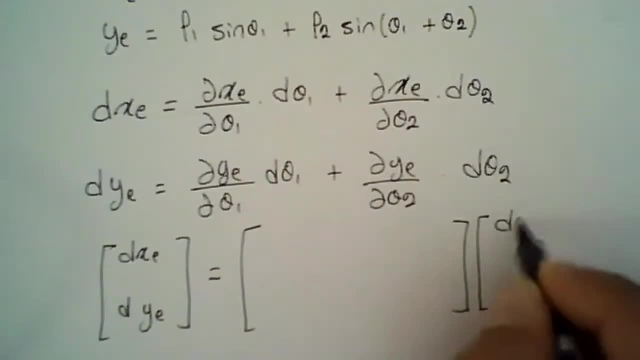 And I can actually put it like that, right. So let's put delta one here, delta two here, right. So these two guys right are being moved like that right. So this is coming like that, right, And then this is coming like that here. 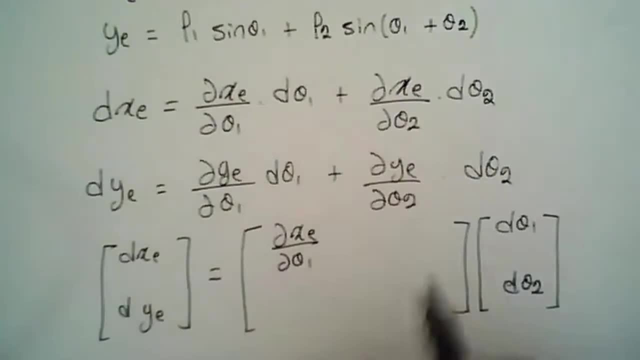 So I can write it like that: Dye Dye right, And then I have Dye Dye right, And then here I have Dye Dye right. So now I can actually, you know, to summarize this: 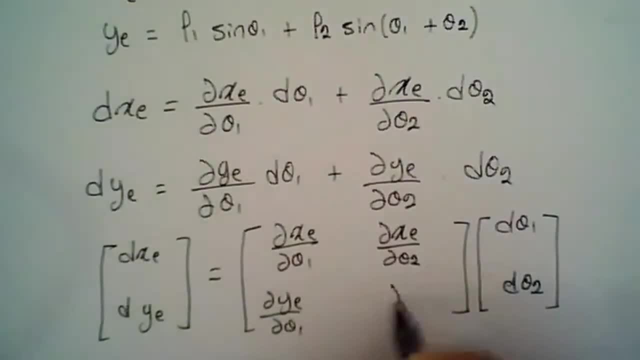 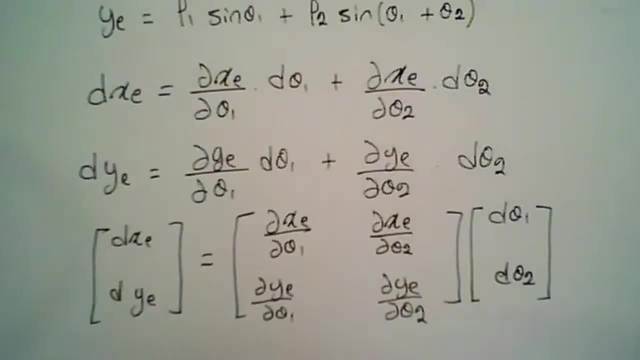 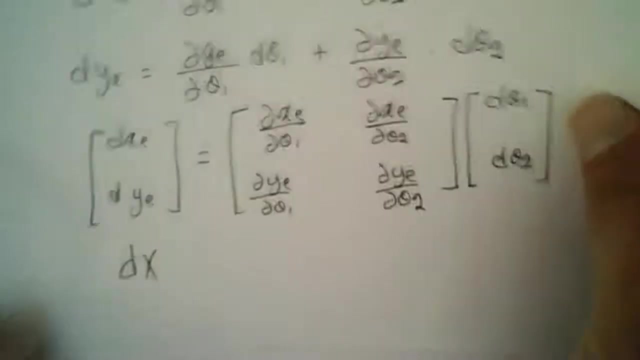 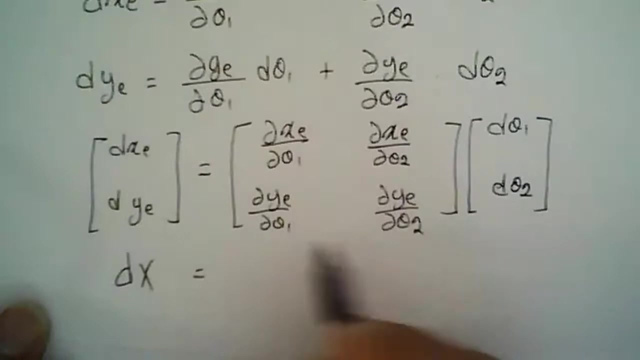 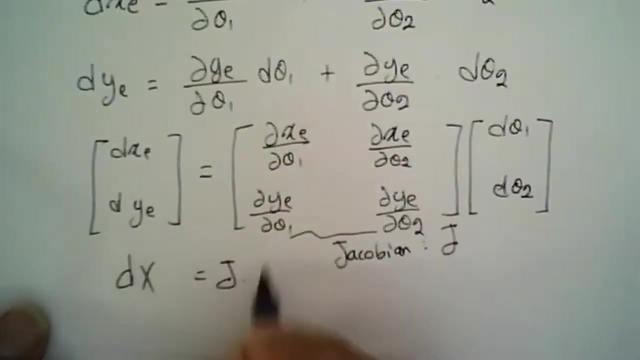 I can actually write this guy as dx. I can write this as dx is equal to, so this guy, basically, is actually called a Jacobian. so this is a jacobian of the robot and it's referred to as j. all right, so dx is equal to j. 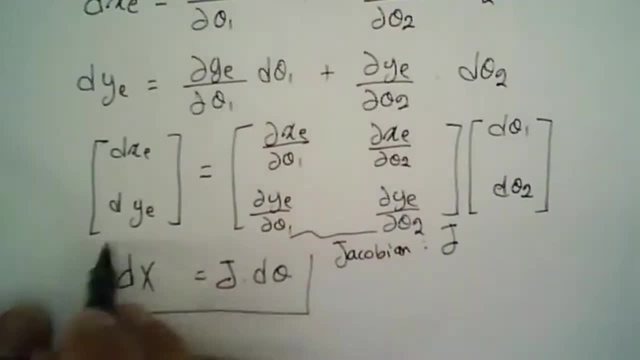 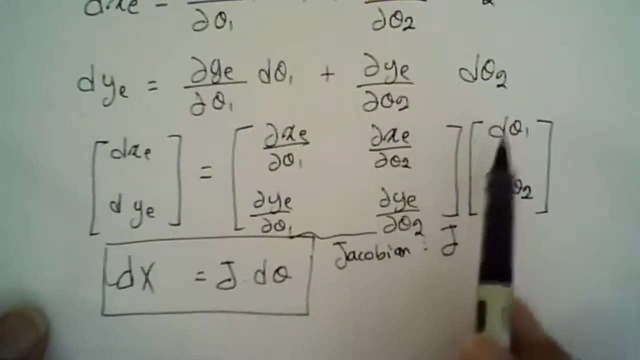 d, theta, and this jacobian matrix actually allows me to relate any small variations of theta to any cartesian variation of the robot, right? so we know j is going to be a function of what j is actually a function of, theta 1 and theta 2, right? why? because x, e and y are both functions. 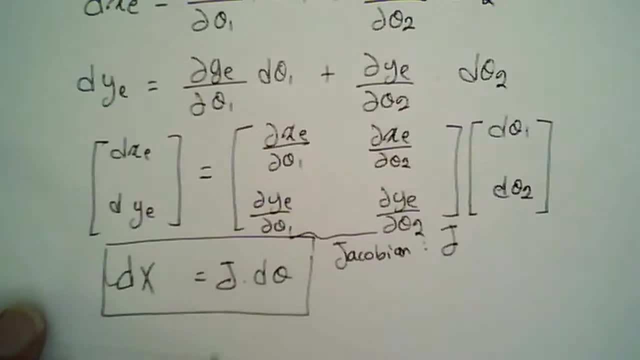 of theta 1 and theta 2. so j is a function of theta 1 and theta 2. so for any given pose of the robot or for any given you know if, for any given values of theta 1 and theta 2, right, if i? 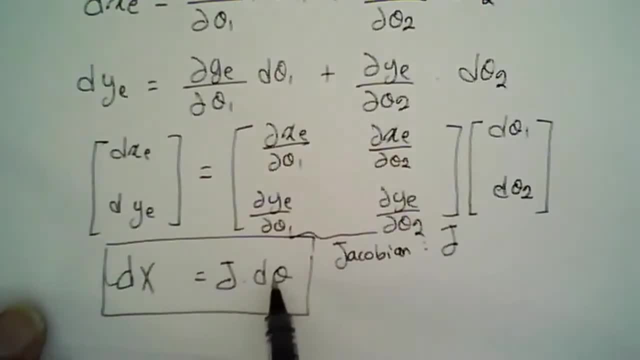 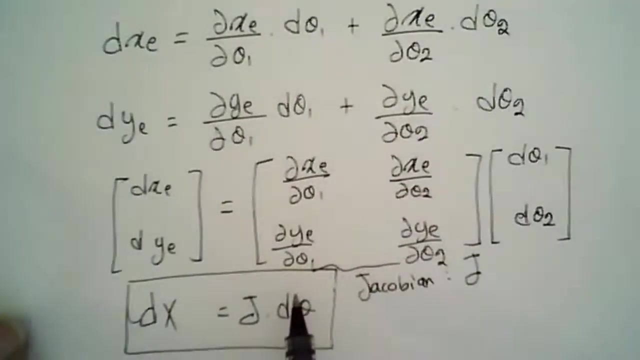 have. i can calculate the j and i can calculate, if you know that does move by. you know this guy by one degree and then this guy moved by, you know, minus one degree. i can actually relate dx, all right, um, we're going to do actually an example now. uh, very quickly, but what is also 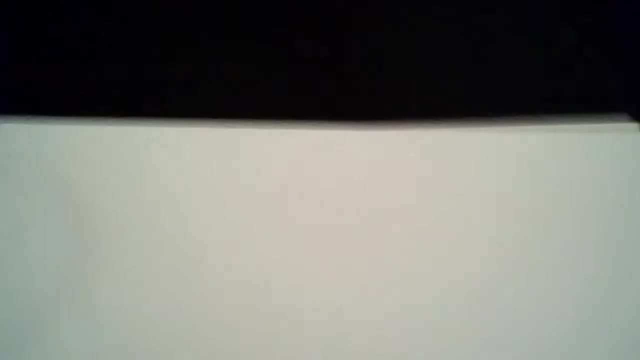 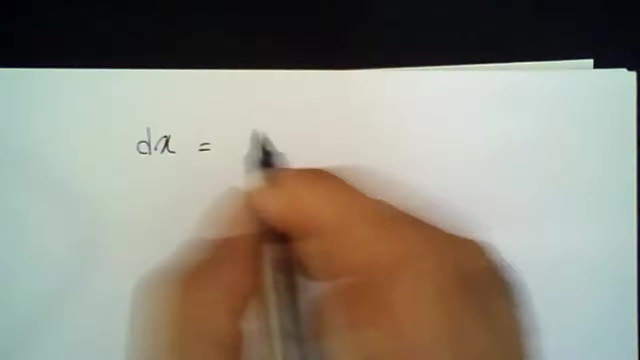 very important here to have is. so now we can basically relate, you know, small movements in the cartesian into small movement in, uh, you know, the joint space of the robot, right? joint space is where the tetas are existing and these are vectors, right? so dx is, you know, x, y, if you have. 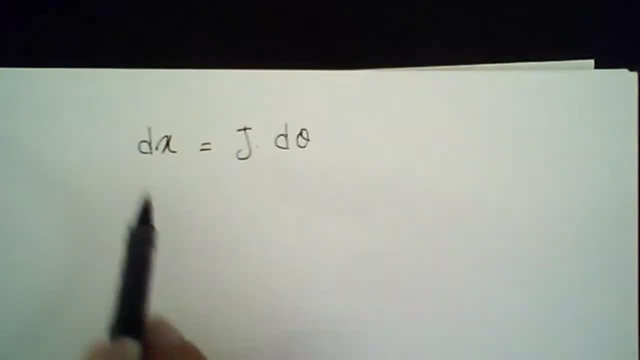 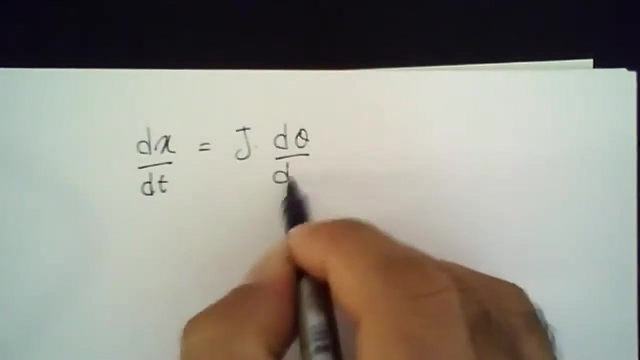 you know more than two degrees of freedom. it would be x, y, z, your patrol, for example. ultimately, in this course we're not going to be dealing with that, so we're doing mostly two or three degrees of freedom, robots. what i can actually do is i can now differentiate with respect to dt. 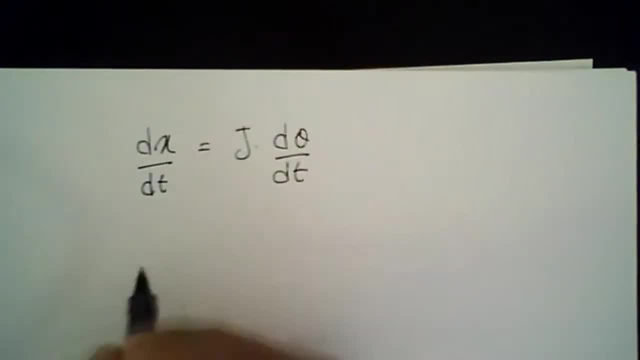 right. so if you divide by dt on both ends, what do you end up with? so this is actually the velocity of the robot, which is the velocity of the robot, which is the velocity of the robot which is the right. So the Jacobian also relates the velocities. 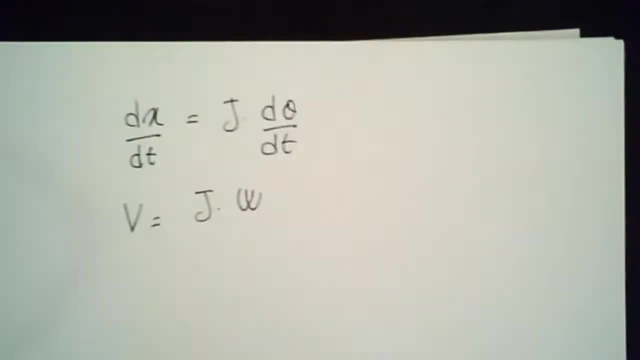 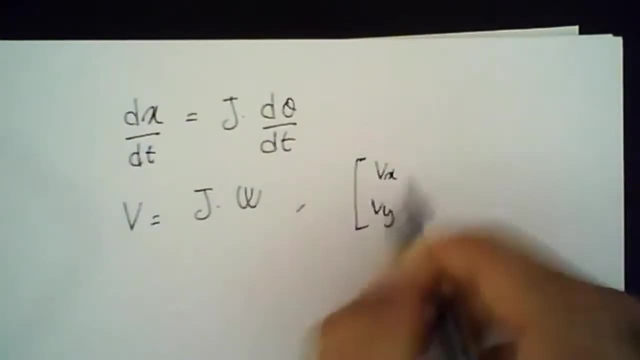 And then, what is d, theta d? t Is your angular velocity vector, right? Well, what is d? d is actually equal to? what Is equal to vx, vy, right? So here we are dealing with vectors j. What is your omega here? 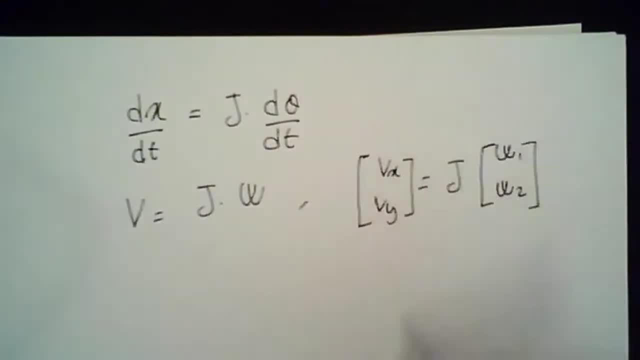 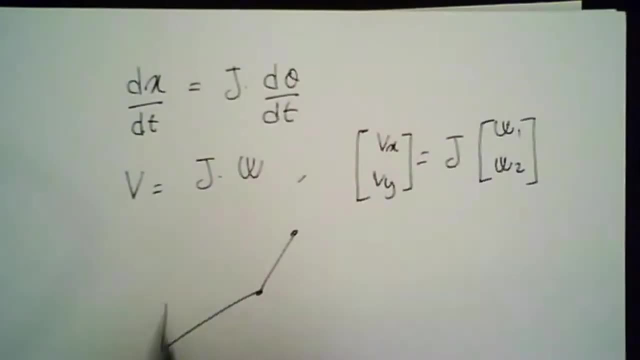 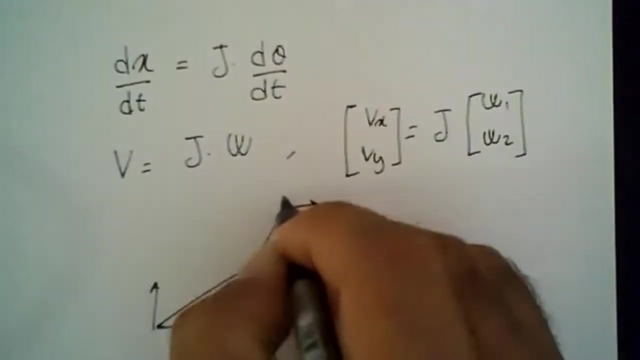 It is omega one and omega two. So if I actually so back to my previous robot, this is what I had. So what is the Jacobian doing? basically? The Jacobian is actually relating is rating. this is the x velocity of an independent factor. 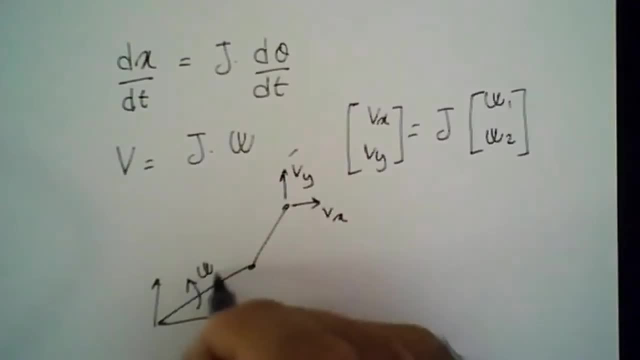 This is your y velocity of an independent factor. This is omega one And then this is omega two. Remember, omega two is not absolute right. Omega two is only relative to omega one. If you want to get the net velocity of this thing, 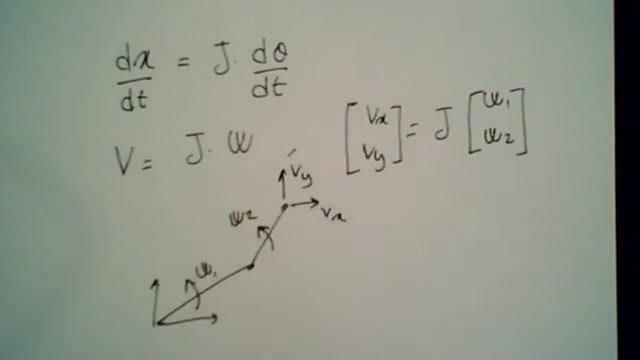 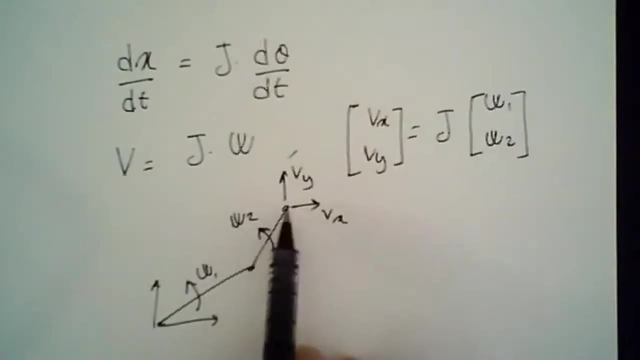 like the angular rotation of this thing. you have to basically sum omega one and omega two, okay, So this is a very important relationship that Jacobian establishes between the Cartesian velocities of the independent factor and the rotational velocities of the various joints around the robot. 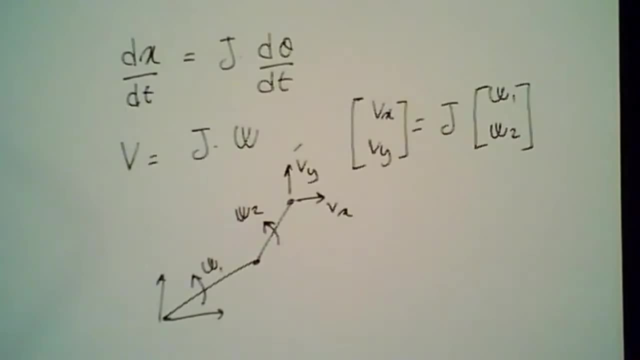 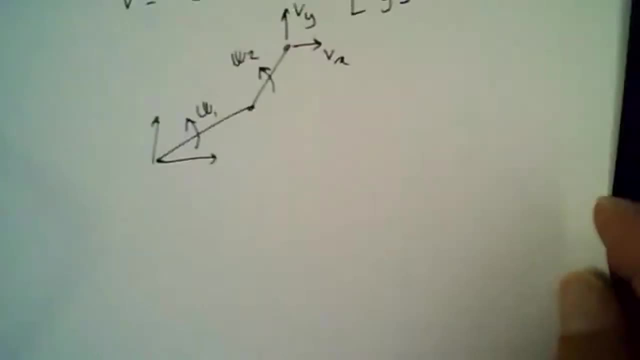 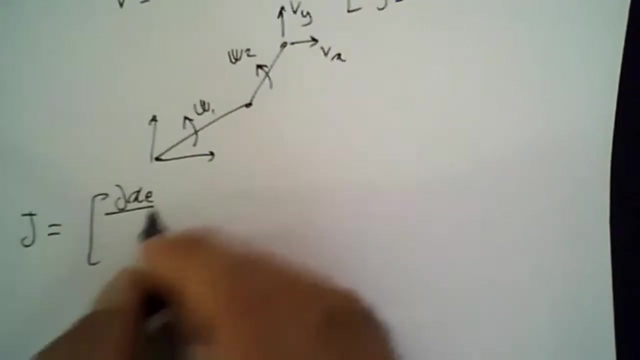 Okay, what I would actually like to do now is let's actually go ahead and then solve the Jacobian and then continue to work on the Jacobian. And we said the Jacobian is gonna be provided to us as well As As g x e d theta one, g x e d theta two. 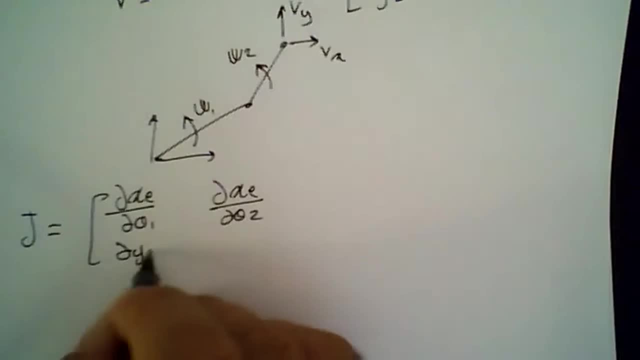 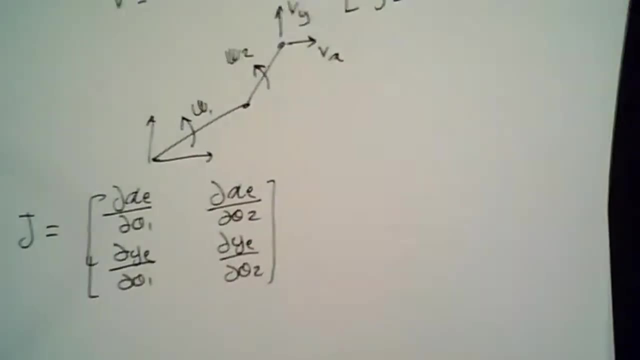 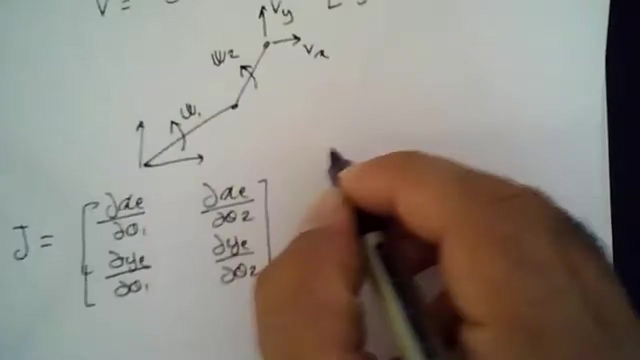 and g y e d theta one and g y e d theta two. Okay, how do I calculate g x e d theta one? So let's do it here. So g x e d theta one, g x e d theta two, That's gonna be equal to. 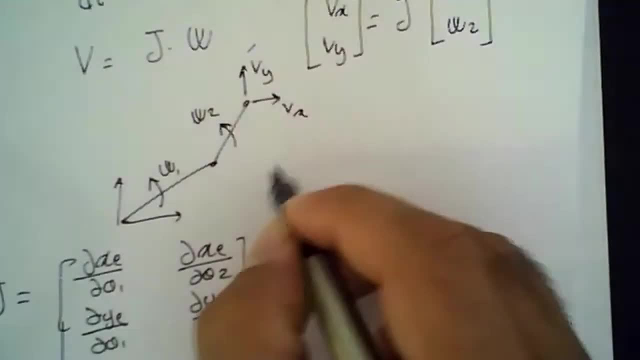 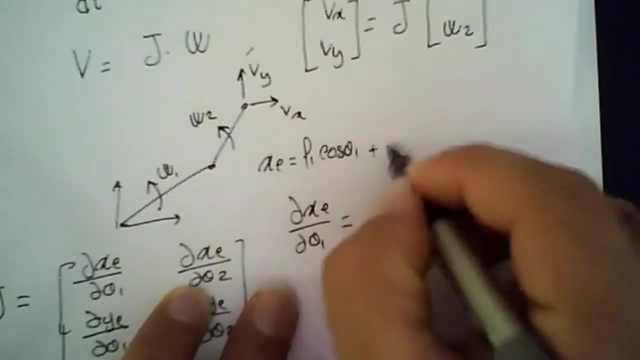 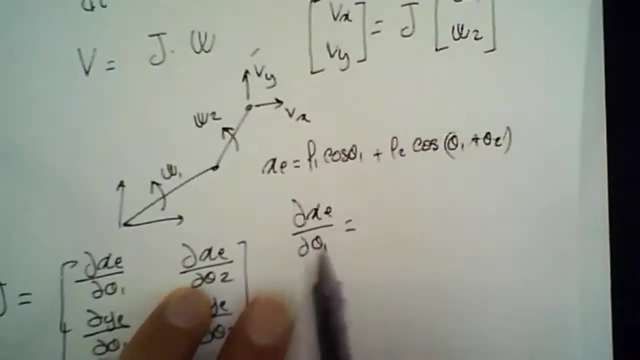 well, I'll quickly rewrite what was x e. So x e was equal to l one cosine theta one plus l two cosine theta one plus theta two. So g, x e d theta one. basically we are doing the partial derivative of x e. 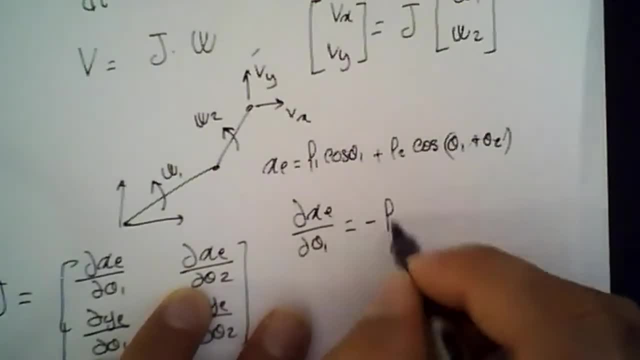 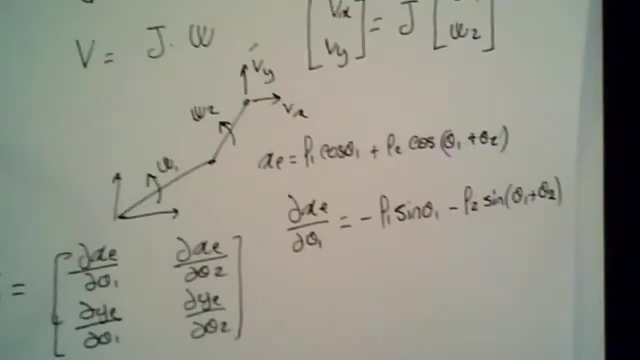 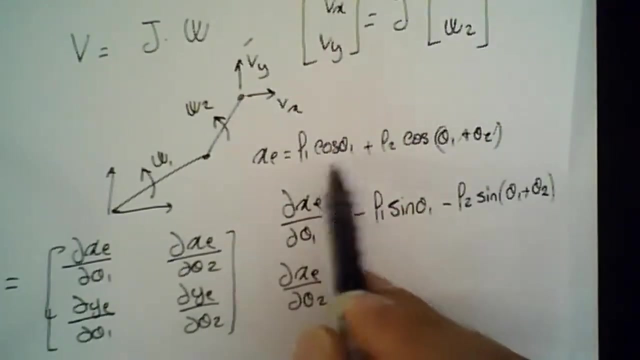 which is theta one, right? So this guy is gonna be minus l one sine theta two, Theta one. And then here, minus l two sine theta one, plus theta two, right. How about g x, e, d, theta two. Well, this guy is gonna be zero. 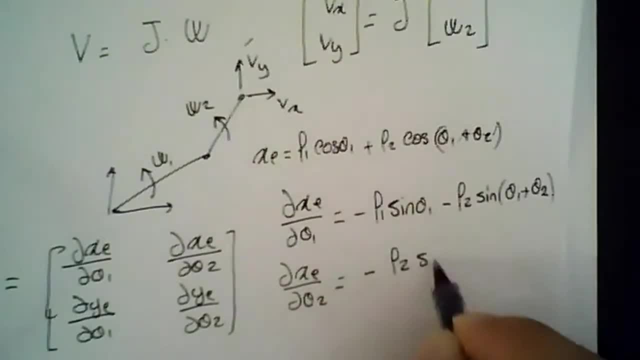 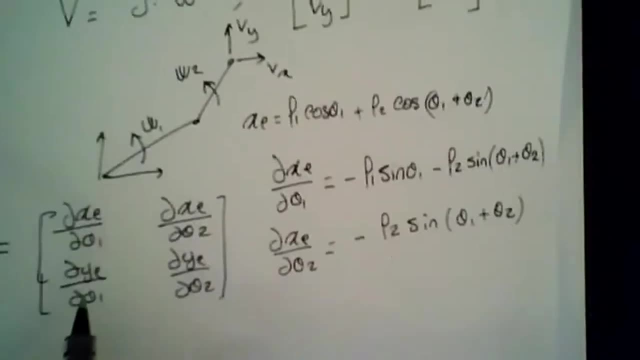 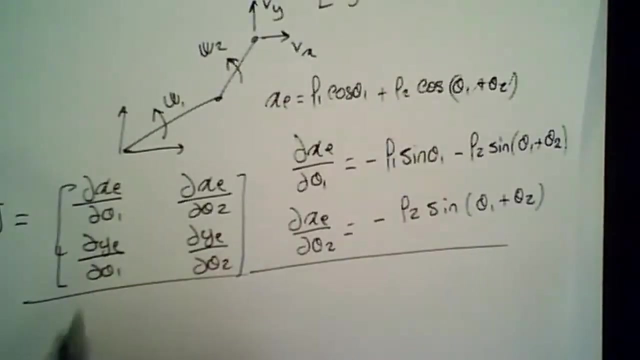 This guy is gonna be equal to what Minus l two, sine theta one, plus theta two. Now let's continue here. So what was? So we need to get d? y e d theta one. So we recall that y e was equal to. 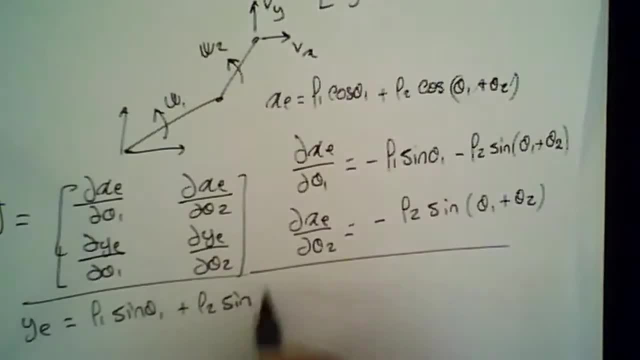 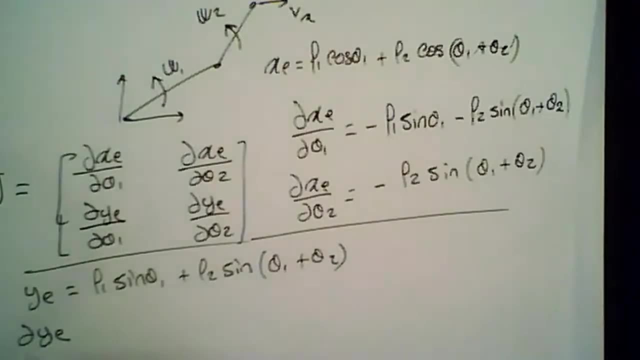 l one sine theta one plus l two sine theta one plus theta two. So we need to capture d y e in terms of d theta one. So it would be l one cosine theta one plus l two, cosine of theta one plus theta two. And on the last term that we are calculating, 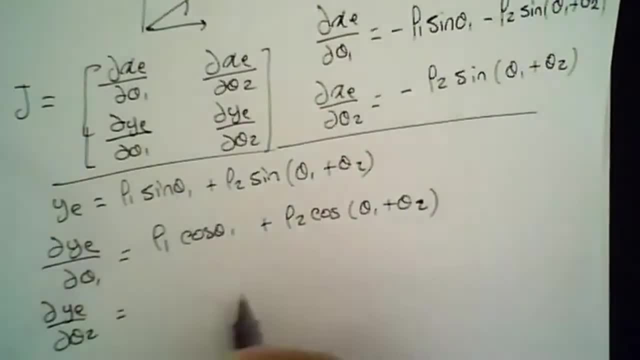 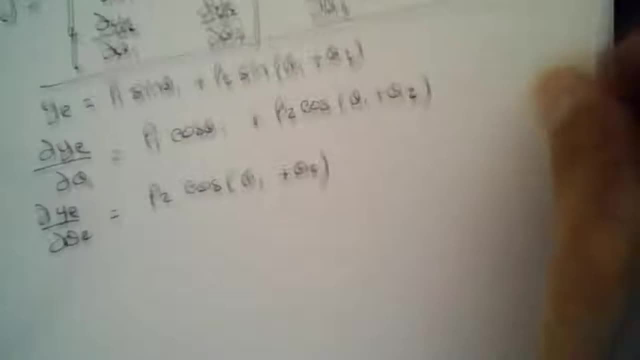 it's gonna be equal to UYE delta two, which is equal to what L2 cosine of delta one plus delta two. So the Jacobian for this two degree of freedom robot is given Q, as what First entry is the XE E delta one. 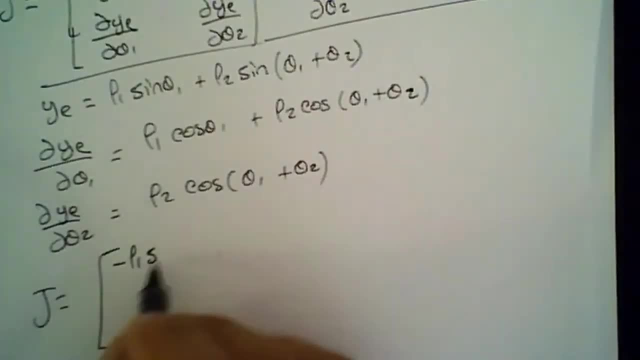 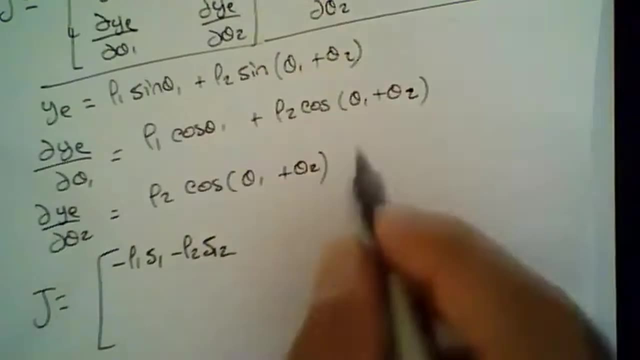 which is equal to minus L1.. So I'm gonna do sine delta one as simply S1, minus L2, S1, 2.. Okay, Now the XE delta two is equal to minus L2, S1, 2,. 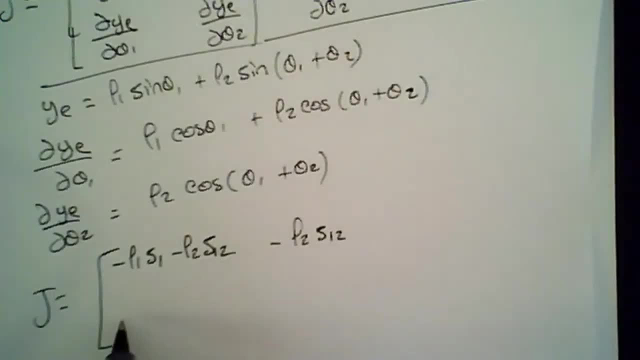 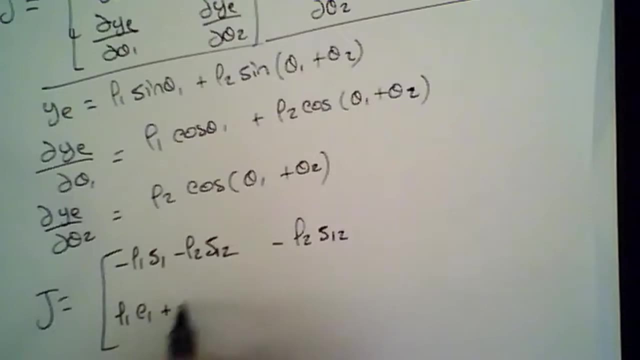 which is sine of delta one plus delta two. The second row is TYE delta one, which is equal to L1, C1 plus L2, C1, 2.. And then I have TYE delta two, which is equal to L2, C1, 2.. 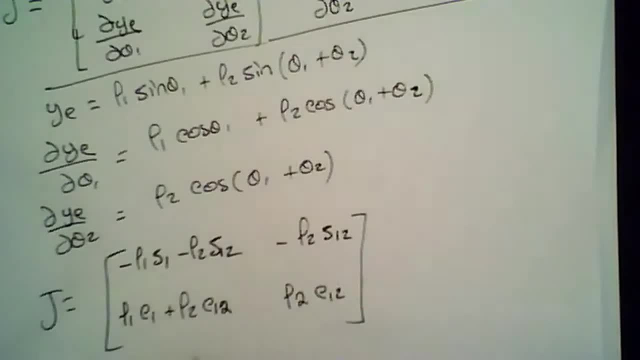 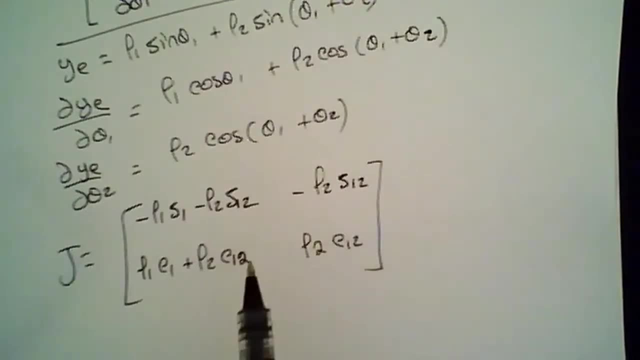 So now you can see, basically, the Jacobian is a two by two matrix in this case. And the reason why it's two by two, it's because it's a two degree of freedom robot. right, It's a two degree of freedom robot. 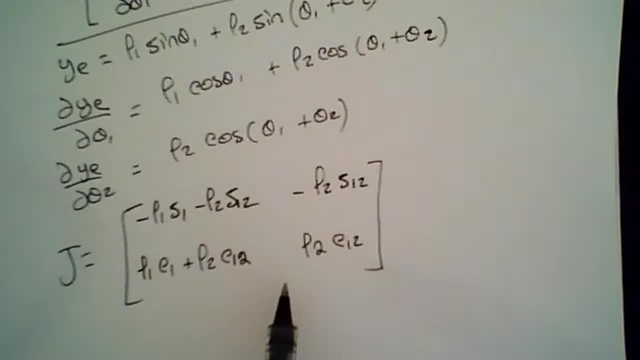 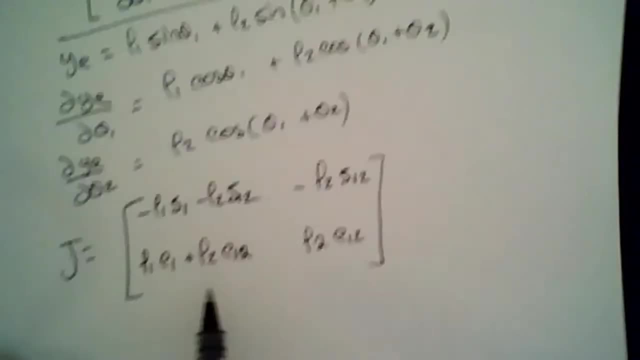 and it's operating in a Cartesian space. right, That's operating in a 2D space. That is why this guy is a two by two. We'll actually go more into this as we go later in the course, But you know this is a Jacobian. 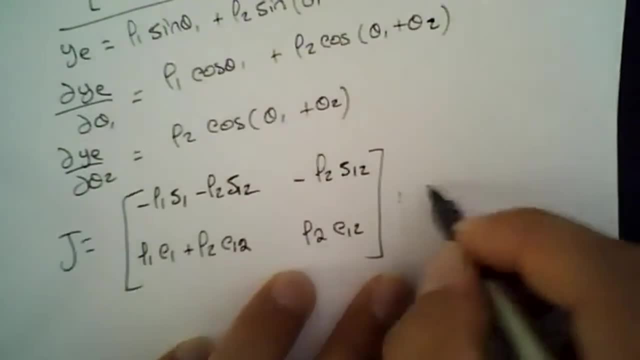 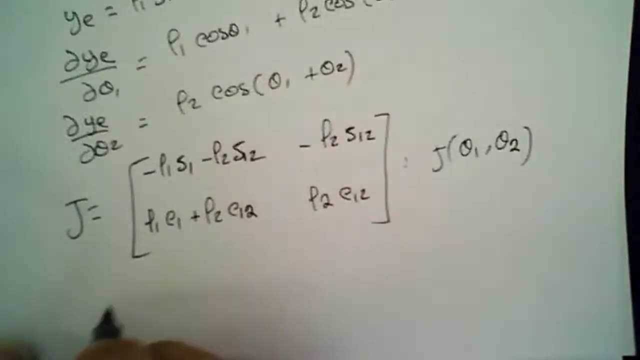 and now the Jacobian is actually a function of J, is a function of delta one and delta two. right, It's not a function of XE or YE. So now back to my relationship. I know that DX is gonna be actually equal to J delta. 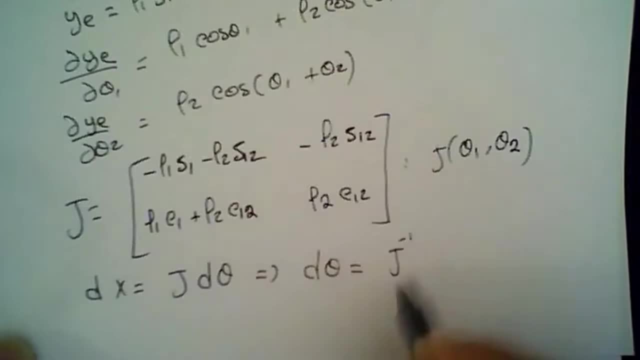 I can actually now solve the delta, which is the inverse of this Jacobian matrix multiplied by DX. okay, So now I can also relate a change in the X with J With respect to a small change in the delta. Now I can actually use this to be able to. 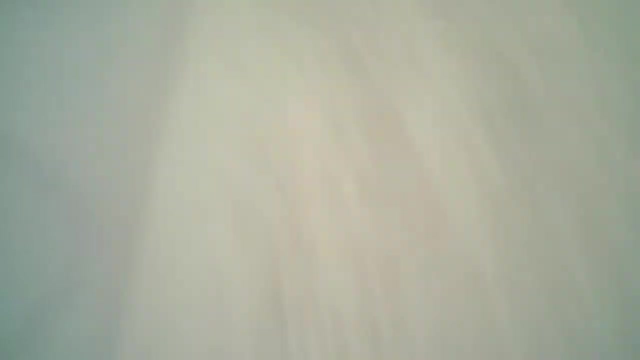 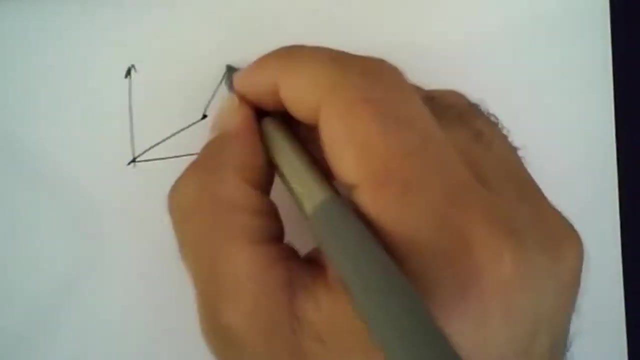 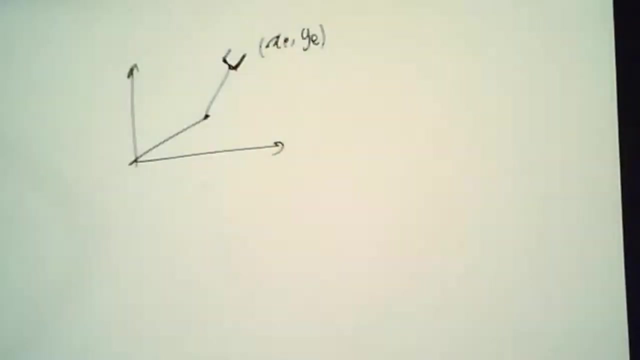 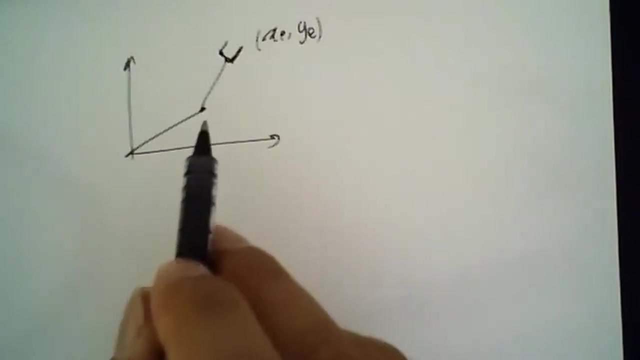 solve the inverse kinematics of the robot, And the way that we will actually do this is based on that right. So let's say you have now this is your robot. So what I can do now is I can actually use my previous relationship to iteratively solve for. 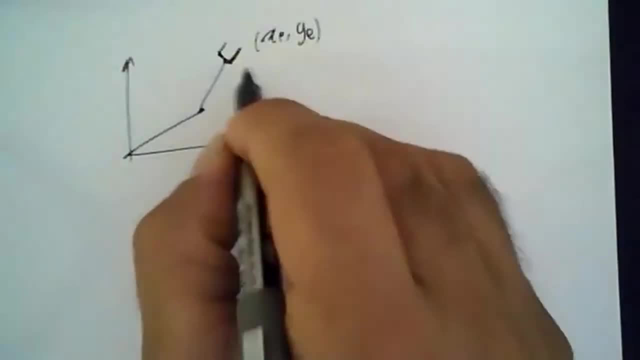 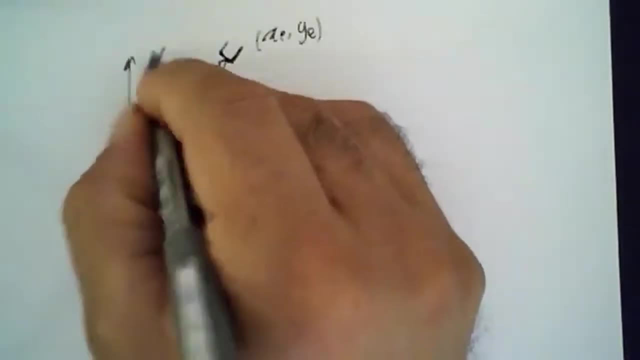 you know the inverse kinematics of the robot, right? But that would be done basically iteratively. So let's say the robot is initially at this, at a particular position, right, XO, which is given to me as X, zero, Y, zero, right. 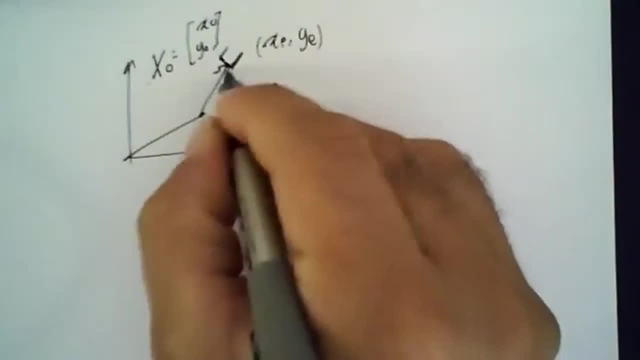 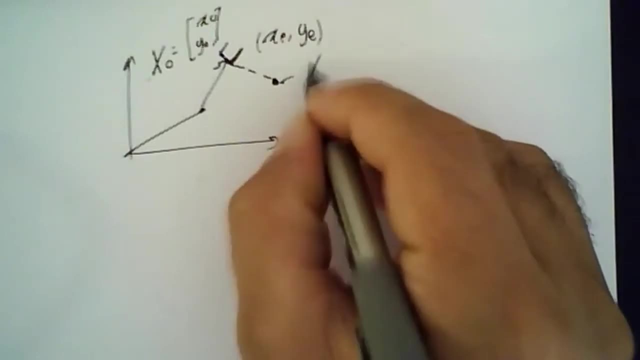 And now I would like to actually take the robot to. you know, I want to do the inverse kinematics of the robot at this position, right, And I'm actually going to get this to X, XG, X of the goal. 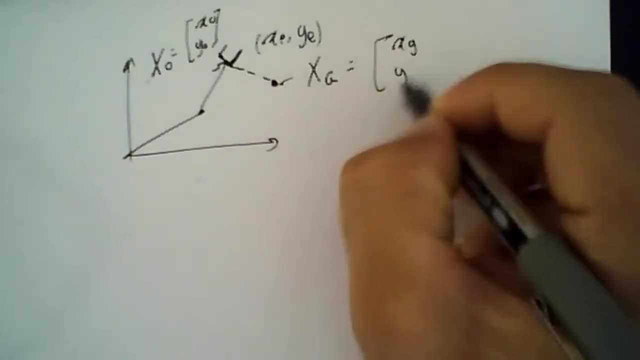 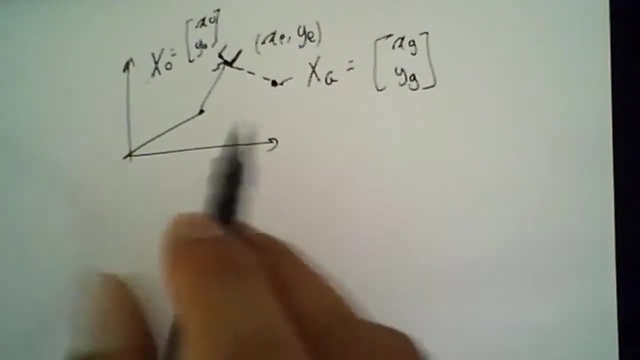 And again X of the goal. basically, as you know, XG, YG. okay, So here's what I can do. okay, So I can now iteratively actually use differential kinematics to be able to solve this problem, And here's what we'll do. 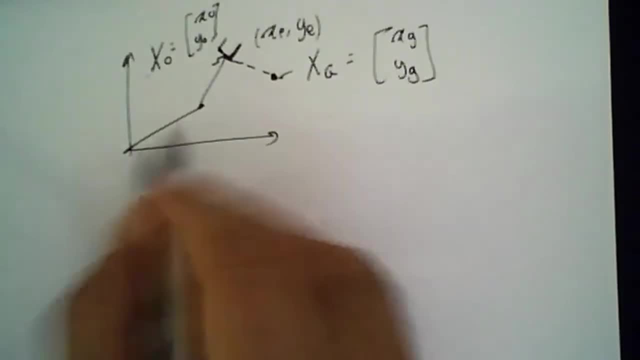 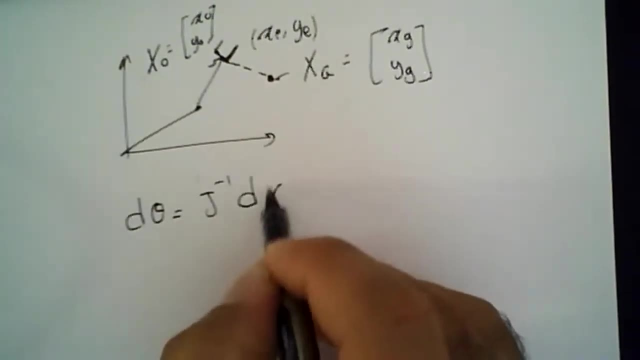 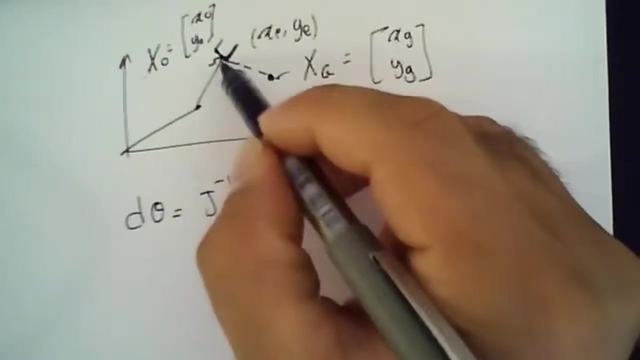 So we know that, we know that the teta right- Small changes in the robot joints- is related by the inverse of the Jacobian with respect to the X correct. So if an angle, basically if the robot is here, and if this and the factor, 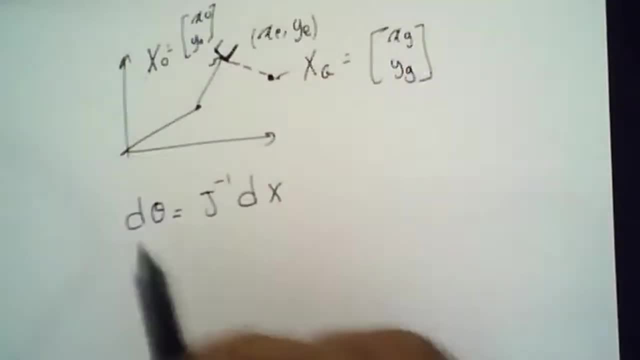 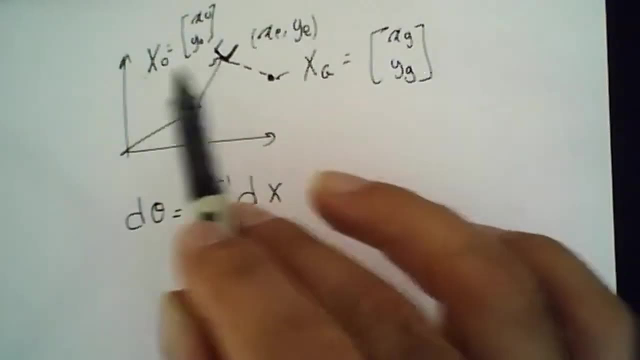 let's say the robot is at this point X zero. basically right, I cannot actually solve teta, what teta one and teta two are for this, but I can actually solve if X zero moves by a little bit. so you know, X zero plus the TX. 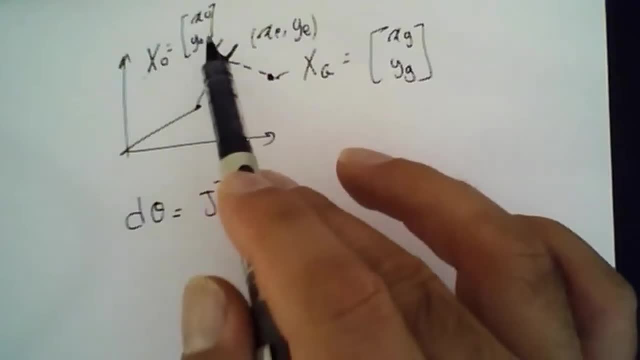 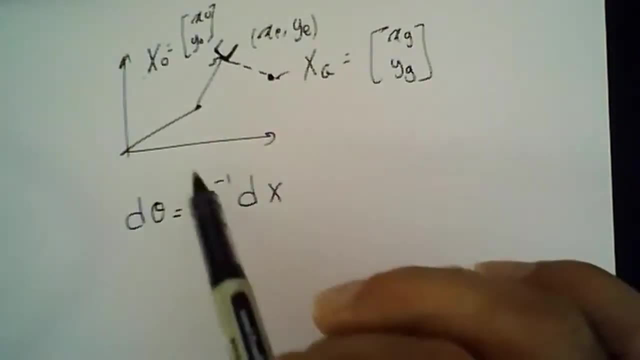 and if Y zero is moved by Y zero plus the Y right, I can do this subtraction like the X and the Y from this point And I can multiply this by inverse of the Jacobian right For these angles and then I can actually solve for how much these joints. 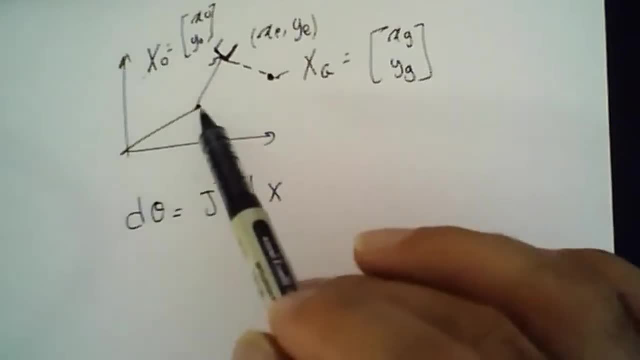 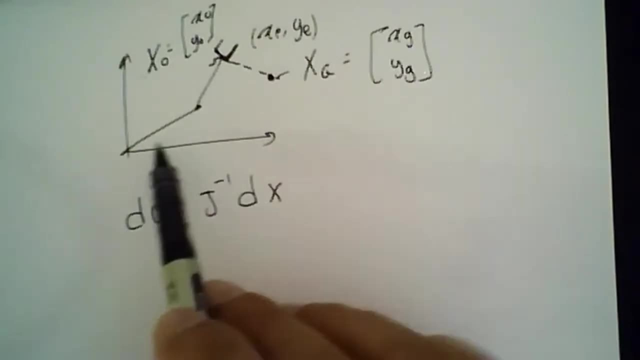 have actually moved. So I know that teta one has moved by the teta one and I know that teta two has moved by the teta two. right To be able to work with the Jacobian actually always need to actually have the angles of the robot. 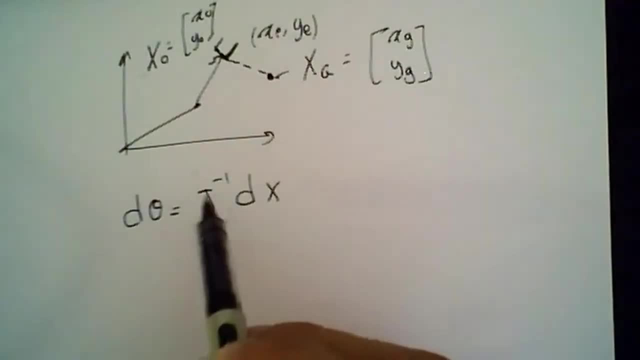 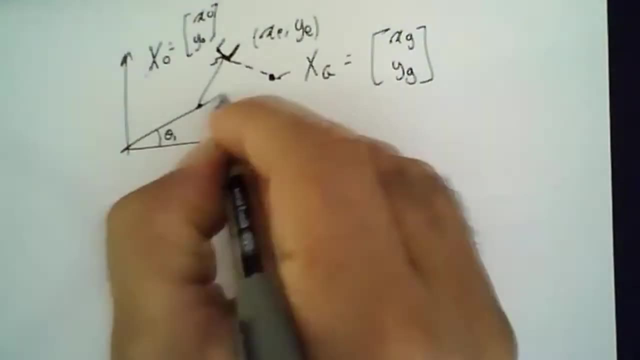 So here is what we will do And here basically, you will have the angle iteratively, So you need to know the initial teta zero here, teta one and teta two. So you would need to actually know that. 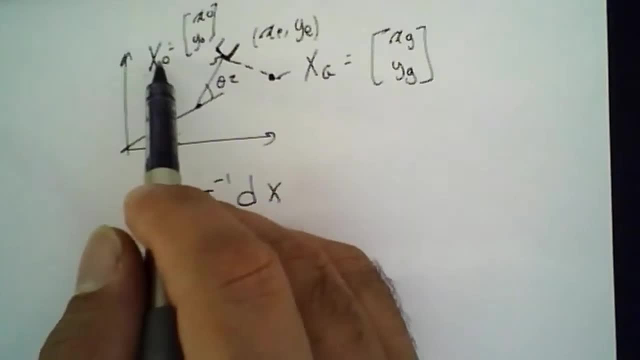 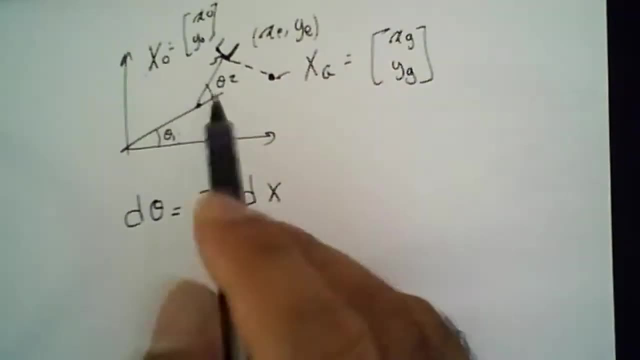 and you use your forward kinematics to be able to calculate the initial collision of the robot, But the solution actually is all developed here in the joint space. Okay, so we always actually have to have that. So let's say we're starting from a random position. 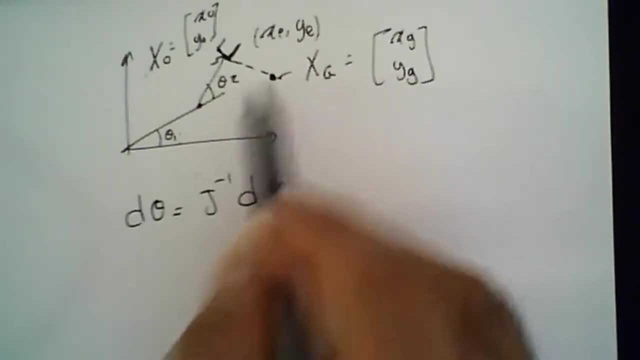 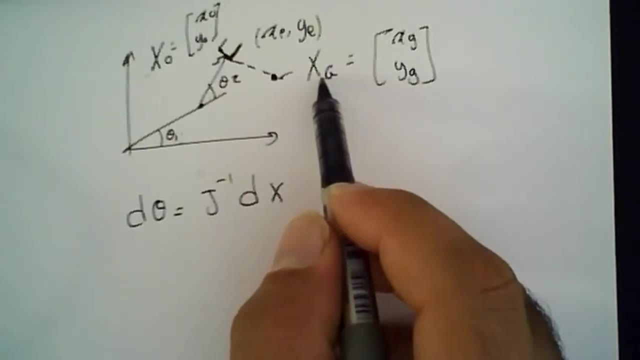 teta one, teta two, and then we are trying to actually solve the inverse kinematics. We are trying to solve, you know, what are teta one and teta two when the end effector is at xg? okay, 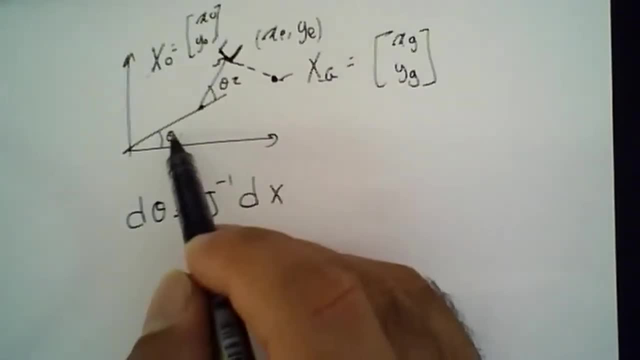 So again, here's the problem that we're solving right: What are the values of teta one and teta two when the robot is at xg? And what we do know? we only know the initial positions or the initial joints positions of teta one and teta two. 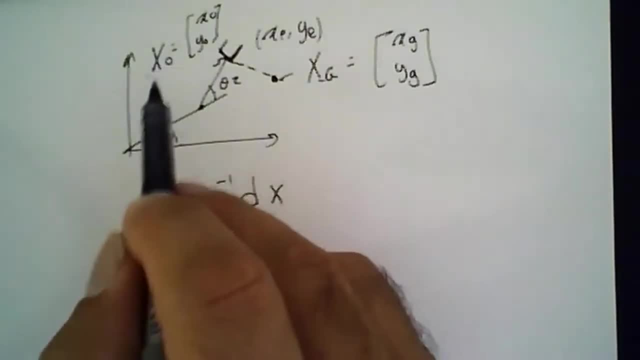 at some random positions. At that random position I'm actually able to obtain the x zero of the robot based on forward kinematics. right, Forward kinematics mean you know what is x one, right, What is x X zero. x zero is equal to l one cosine, teta one. 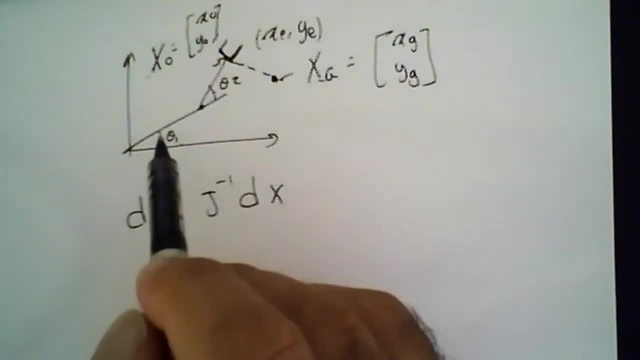 plus l two, cosine teta one plus teta two, And I know y zero is gonna be equal to l one sine teta one plus l two sine teta one plus teta two. right, Okay, deal. So here's what I'm gonna do. 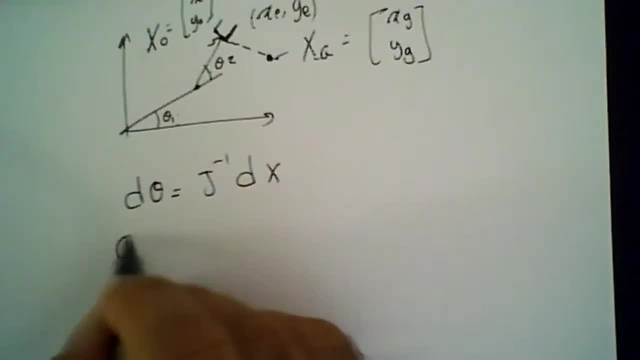 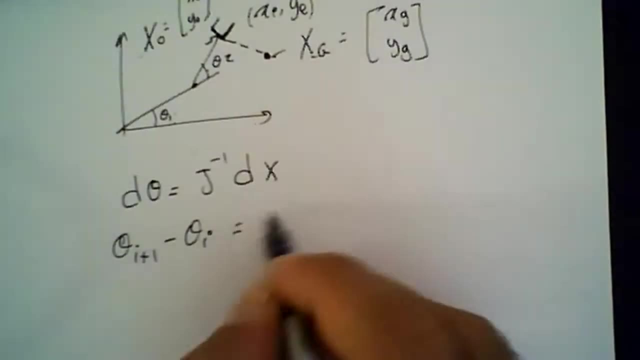 So d teta is actually equal to what Is equal to teta, all right, plus one, minus a pi, Cause we're doing this iteratively right- Is equal to j minus one. What is d x? So d x is basically- I'm starting at this- x zero. 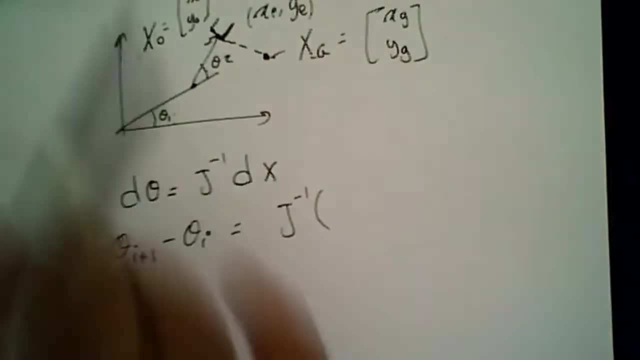 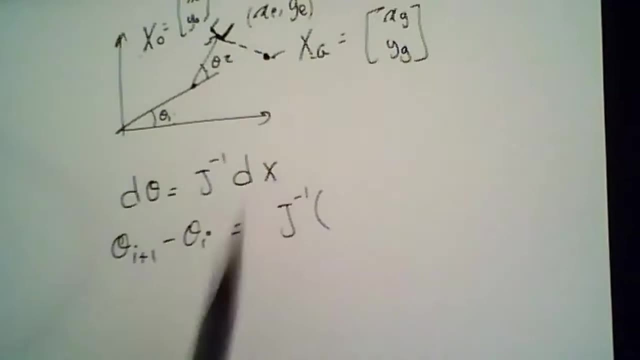 and I'm actually going to this goal position right, But I'm not gonna take this whole thing at one time because it could be a very large d x. We wanna take a very small amount of d x, So we have to actually multiply this by value alpha. 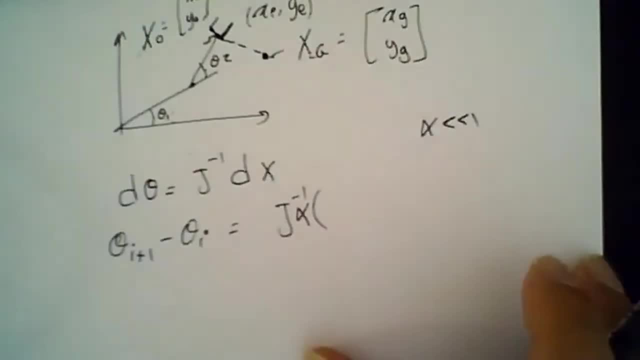 where alpha is. you know alpha is, you know, alpha, much less than one, okay, usually, you know could be like you know 0.01, okay, so so now we're basically multiplying this whole distance by this alpha to be able to reduce this guy, right? so it's going to. 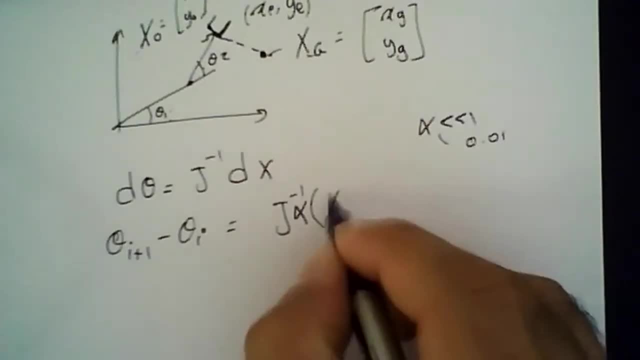 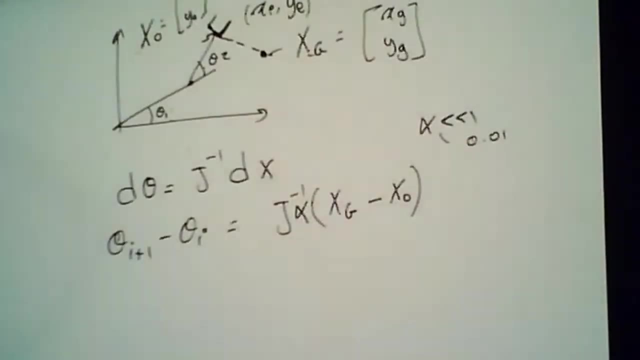 be. what is my dx now? the x is my x goal minus my x zero right x zero is the current position of the robot. yeah, so now i can actually write. so i know my initial tetas right. i know j is a function of my tetan. i can actually now solve for my next step. so this is my theta. i plus one is equal to: 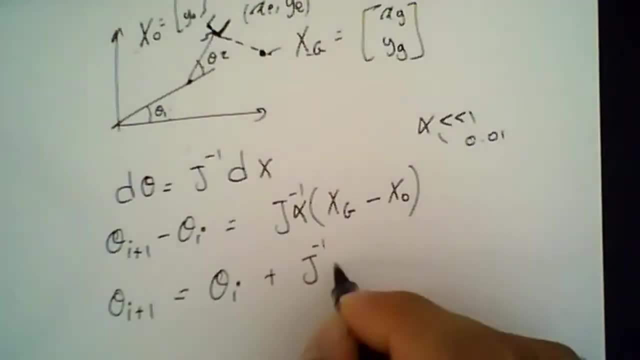 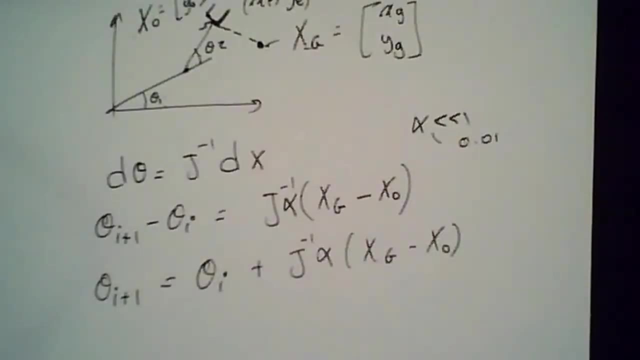 theta i plus inverse jacobian alpha x goal minus x, zero right. so you do that in a loop and you continuously repeat that until your error becomes zero right. so every iteration, basically you update your x0 right. every iteration you update your x0 and the error is reduced. ultimately, 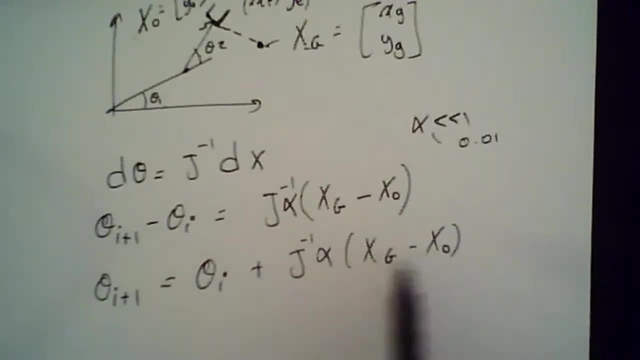 that i will actually convert to one value where you are actually solving the inverse kinematics of xg. okay, how do you get x0? x0 is your forward kinematics right and we know what forward kinematics is by now. it's forward kinematics of your whatever theta i you have. 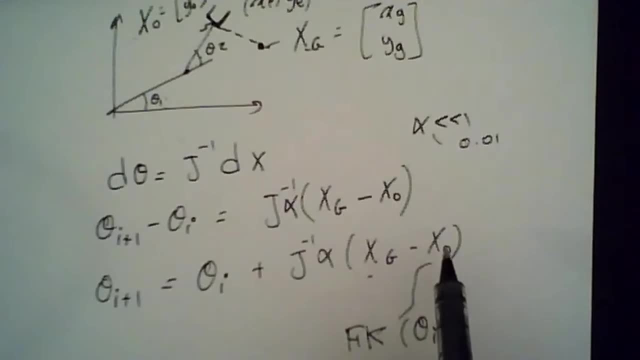 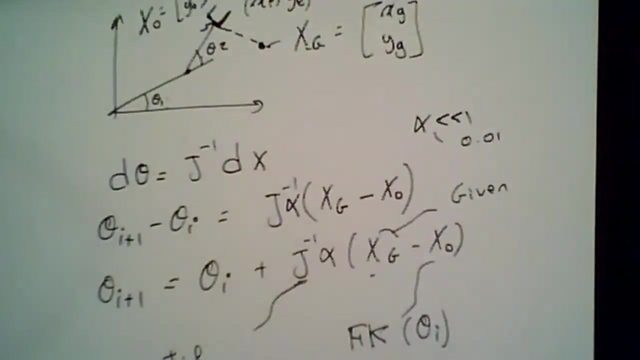 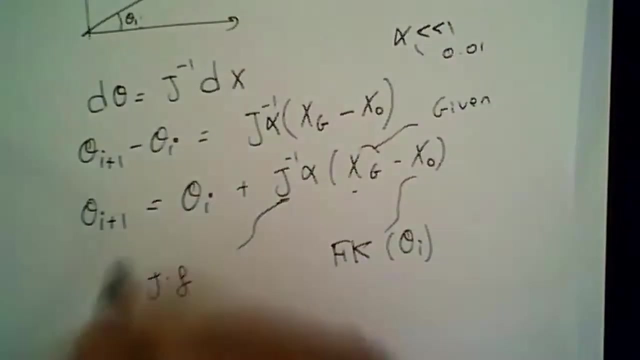 right. so, as you know, the robot basically update your position. does it make sense? what is xg is given to you, right? so this is given, okay. what is j? j is j is actually a function of. let me just stop up here. j is a function of that. i right that i is a vector, right. 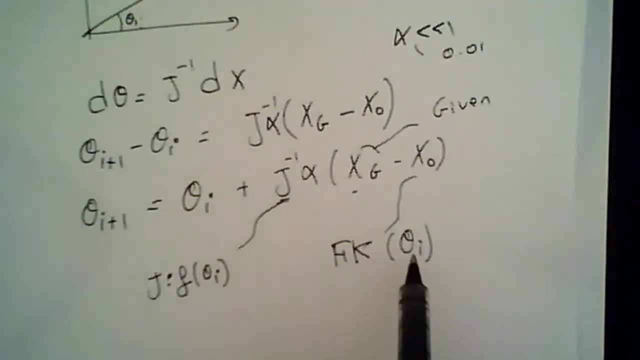 so it's a function of one and two which you actually have it here. so every time you update your data, you compute your jacobian, you update your position and you find your next step down the next iteration. you use this data here and use this data here, right? so always you are using. 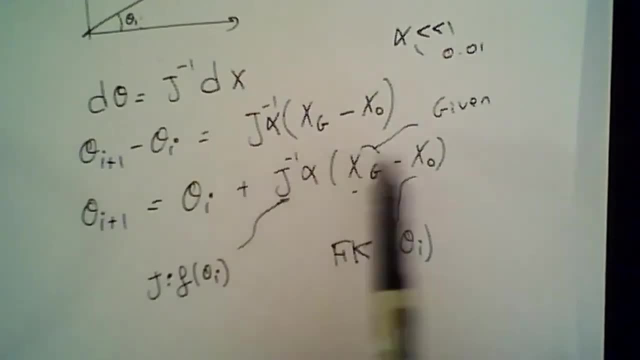 the older capital to calculate your jacobian, to update your position, and you add this increment to your older captain. okay, so i want to give you guys, obviously, some examples on that, and i think the best way to learn that is by really going. so this is how we can do the inverse kinematics of the robot. 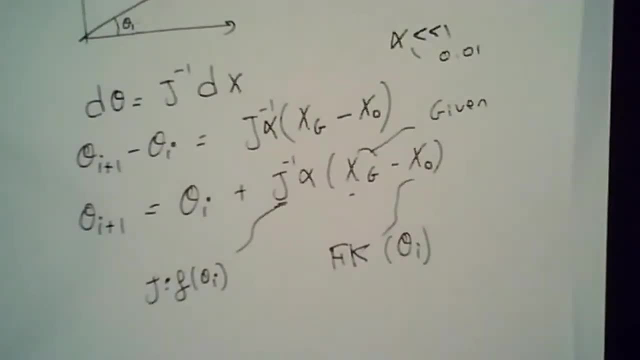 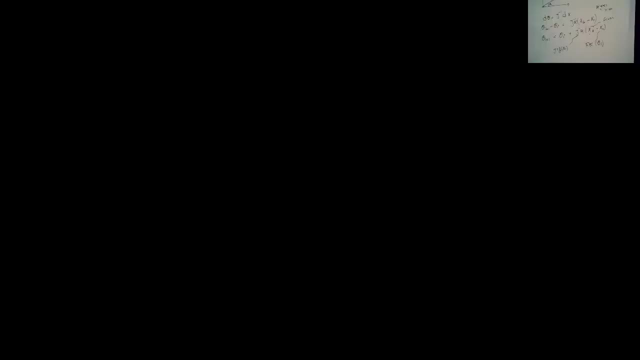 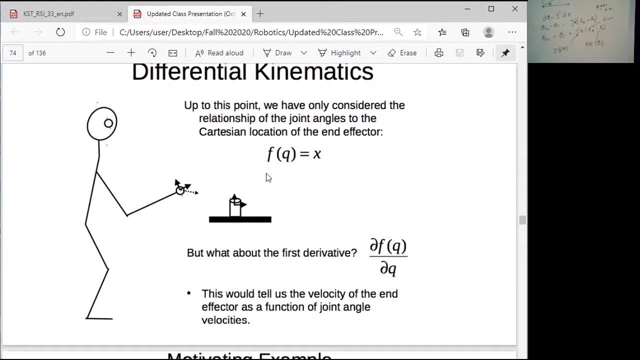 using jacobians, let me quickly share my slide and here i can show that to you guys here. so this is on our note. so this is differential kinematics is called, as you know, uh. x, as is equal to a function of this is forward kinematics, right, um and when. 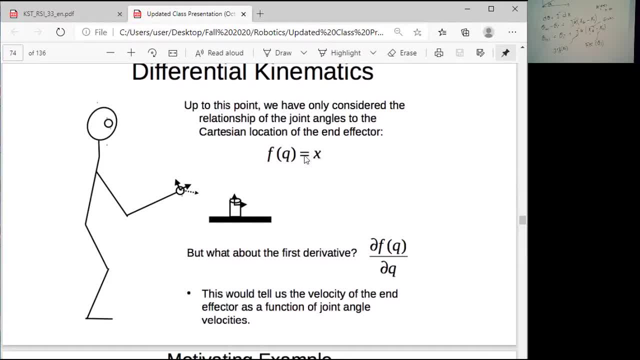 we're trying to find q or the angle as a function of x will be inverse kinematics. uh, solving inverse kinematics from geometry is very difficult sometimes, so what you can do is to actually use differential kinematics. so instead of trying to obtain solving this non-linear, non-linear problem, 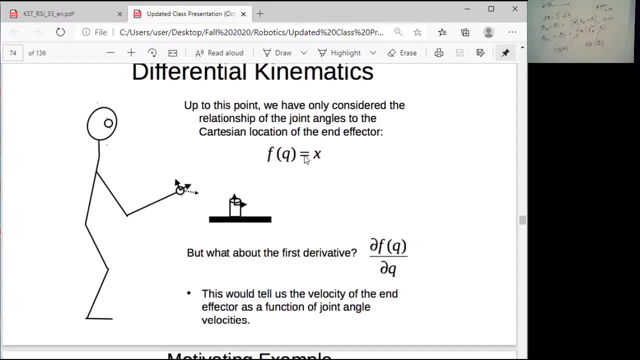 of q is equal to you know, some g function of x for f-4. as you know, this is a non-linear problem. so of x you can simply differentiate forward kinematics, which is very simple. so there is always a derivative for your product kinematics, right for the derivative of the product kinematics. 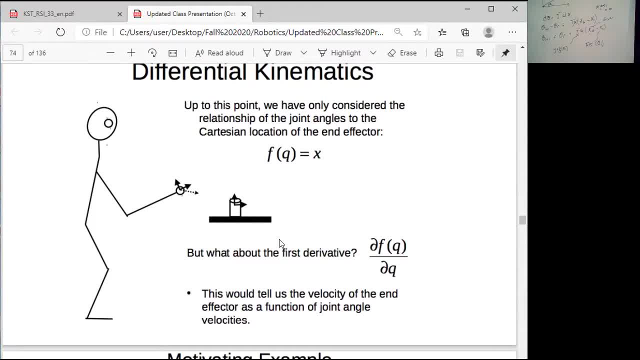 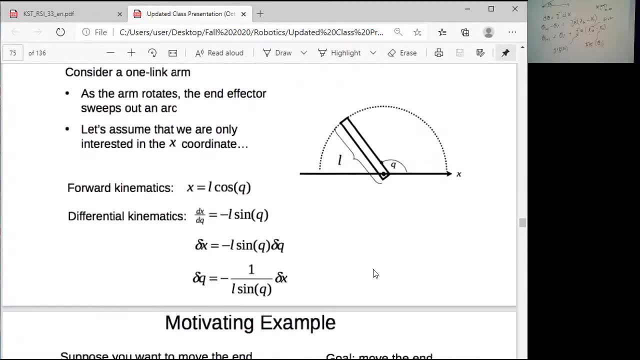 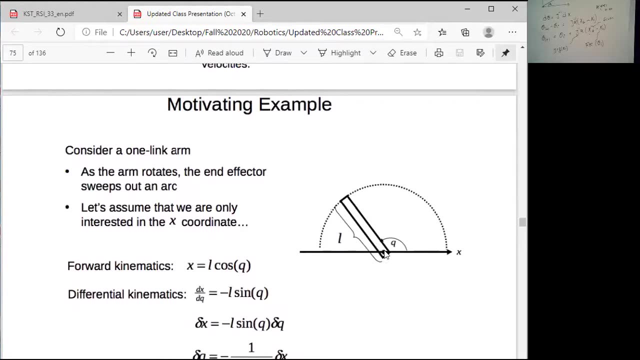 will simply relate, you know, small displacements in the joints to small displacement in the end effector. all right, so this is a very basic example that I have here. all right, so if I have a one degree of freedom system, so I simply have this, you know, bar, and I have the angle: quantum, the forward. 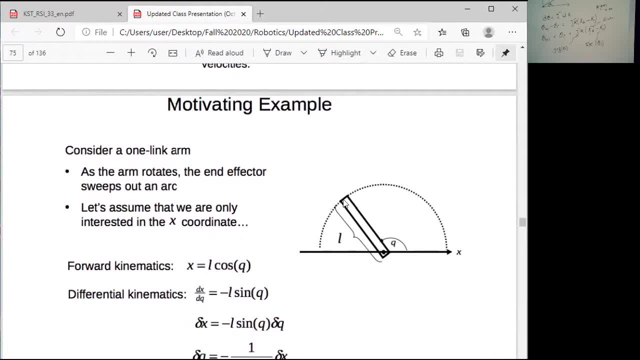 kinematics is basically- I'm locating this position, the end effector position of the function of q, right? so what is the coordinate of the end effector? it will be l cosine q, right? if q is greater than 90 degree, then obviously cosine of an angle that is greater than 90 will actually be negative. so 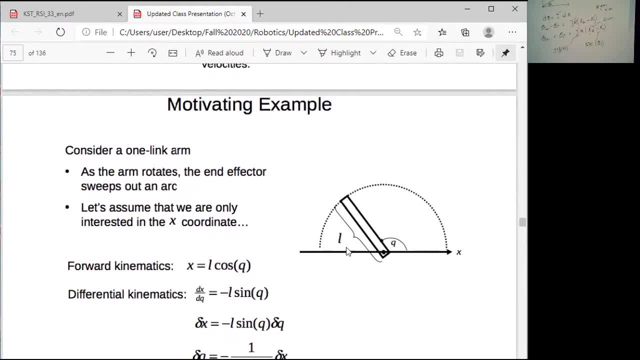 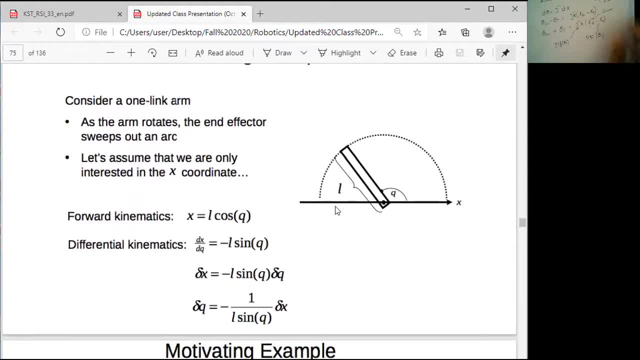 this is my x. it's always valid. obviously, if I want to do the quick inverse kinematics solution, what would that be? so we know here, as inverse kinematics, we know x equal to l cosine of q. inverse kinematics you are trying to find q as a component of x, so q is going to be equal to x over. 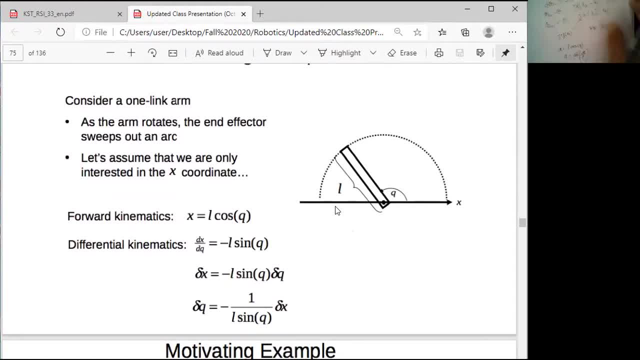 l and you are doing the inverse cosine of that right. it's very simple. but what if you aren't able to see that right? what you can do is you can do kinematics and decide. what you do is you can differentiate the x with respect to teta or dq here. so dx is equal to minus l sine q, dq right. so dq is equal to minus one l sine q. so 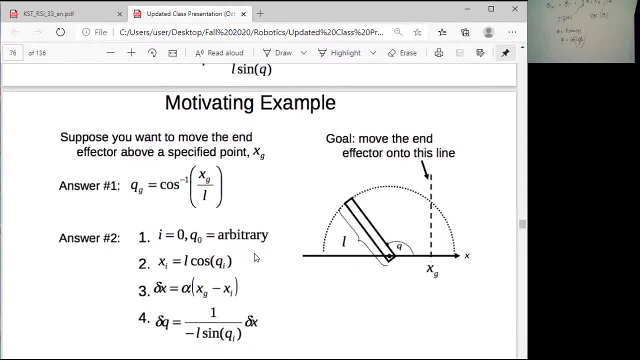 this is basically like a jacobian right apart and one degree of freedom system. so how can we solve this problem? right, obviously, answer one is you do simply the basic inverse kinematics. but answer two is: you start with a random, you know position. you start with square zero, where the bar is currently. 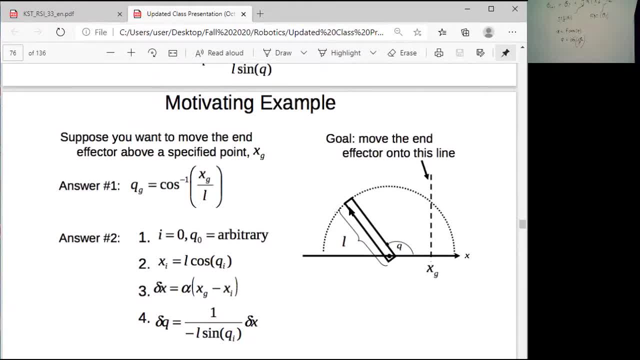 at. if you have a robot, you can pull the encoders right, you know where the robot is based. on the encoders, you can find the position based on the forward kinematics model. then you want to move the robot to a particular point: xg, right, so what is your dx? 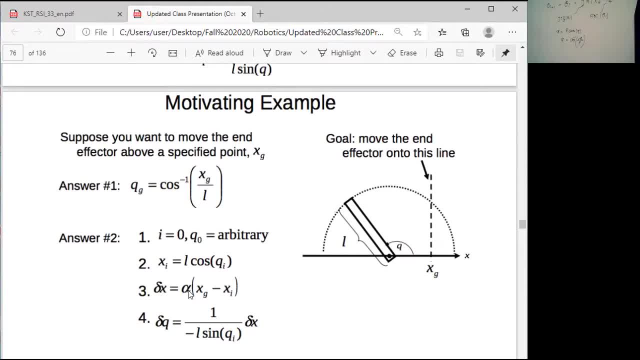 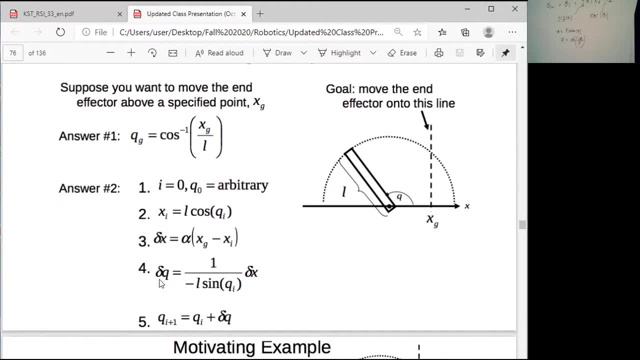 now the x is equal to. you want to take a very small step right. so x squared, minus your current position. once you have the x, you can find the dq right. so what should be the change in the angle that would actually lead you to close down on the error between where you are and where you want to? 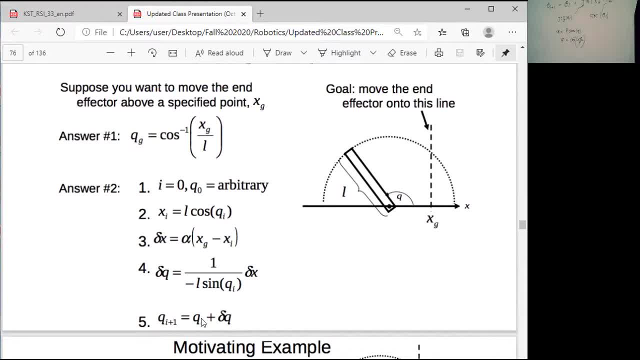 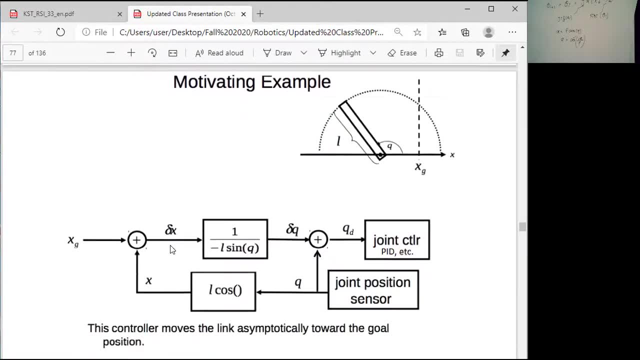 go and then you keep doing that, right, if you keep doing that, ultimately, if you will stop changing, and then the q will actually go to zero because your dx will actually converge to zero. okay, uh, if you- uh, you know, want to visualize that as a, you know, visually, so you, you have a goal position. 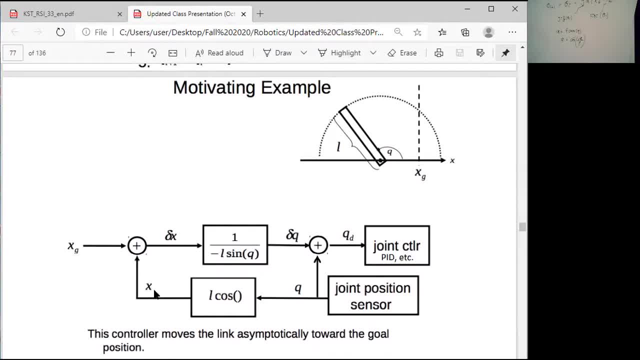 right, this is your current position, just your x goal minus x. so this is the x. so this should be actually a minus. there should be a minus for sure: x goal minus current position. so this is your dx, at the inverse of the jacobian here, right here it's mapped on one degree of freedom. so we have. 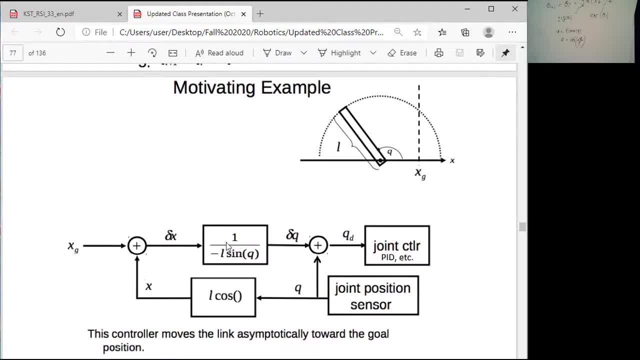 the dq. so remember: dx multiplied by the jacob inverse jacobian will actually give you the q right. so this is your change in the q, but you also have to add that to the change in position to the current uh right. so d theta plus theta will actually give you the latest right. so now we. 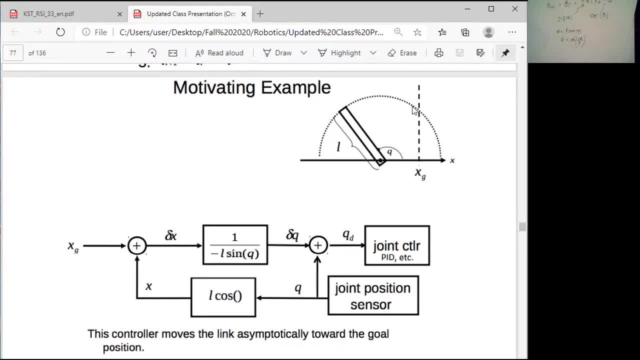 actually have a position where you want to send the robot to. so now you can feed that into your qi controller or whatever you are doing to actually set the position on the actual hardware. okay, uh, this is the loop. so again, this actually has to be minus of one month itself. so xg minus. 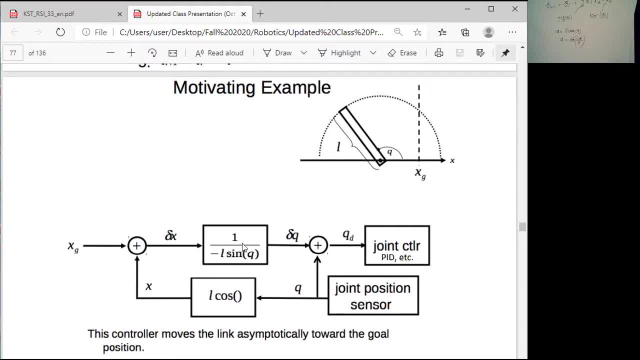 x right will give you dx. dx multiplied by inverse j will actually give you change in tecta right and then change in tecta will always actually be done, be added to your current tecta. so what is that? this is your fk model. right fk model will take. 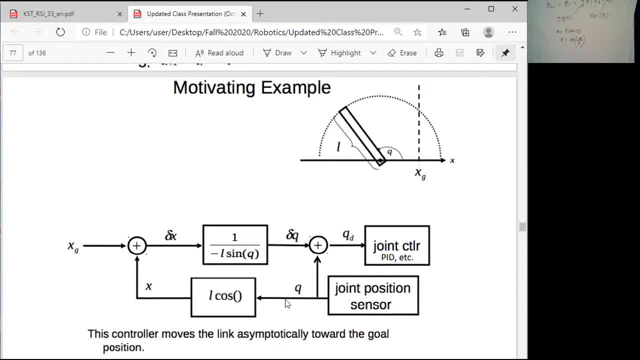 a joint position from the sensor, for example, your joint position will fit them into your fk model and the fk model will return your actual partition position on the robot right. and then xg is where you actually want to take the robot to, where you are trying to command the robot to go to. 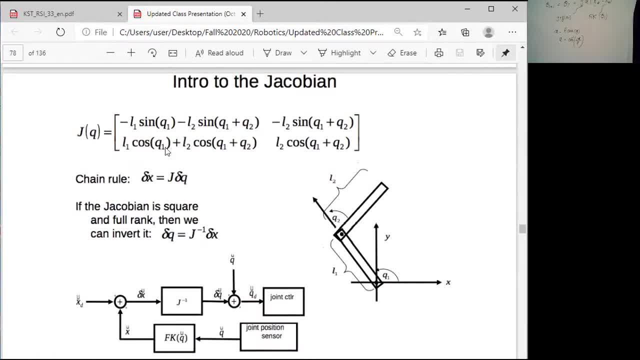 okay, that is that. so on, a two degree of freedom robot. so this is actually what we had earlier. so this is a two degree of freedom robot. we know how we got that right. so you get that by differentiating the core kinematics. respect that the one, and then the 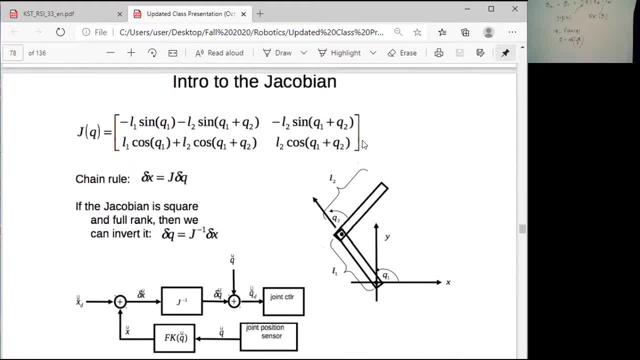 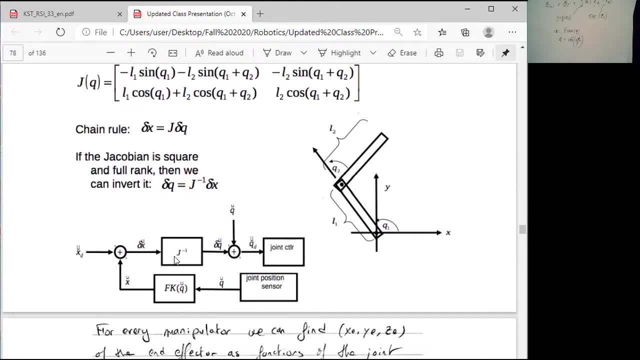 two here, right, this is your x, and then this is along your y, right? okay, so eq is equal to the inverse of jacobian. so this is my inverse jacobian. this is my forward kinematics. so q, you feed that into your forward kinematics in your x position. this is your desired desired. 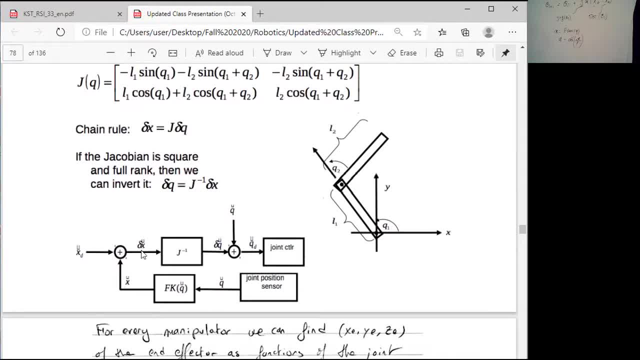 minus existing position will give you the error right. you still have to multiply this by alpha, because here we're doing this on a very, we're moving the robot by very tiny amounts right and uploading the whole thing at the time. so that is why you actually have to have an alpha here. that 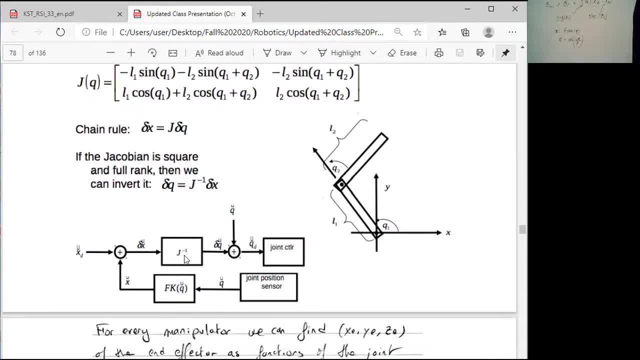 is very small and you multiply this by the inverse of the jacobian, you get how much. you should change that the one, but you still have to. you know that change. that is relative to your current joint positions. so you still have to add that to your current joint position and then you would actually 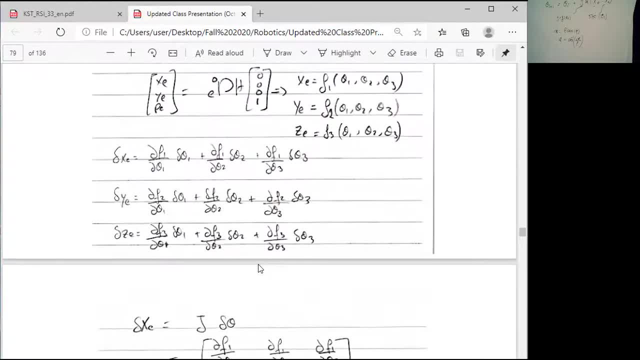 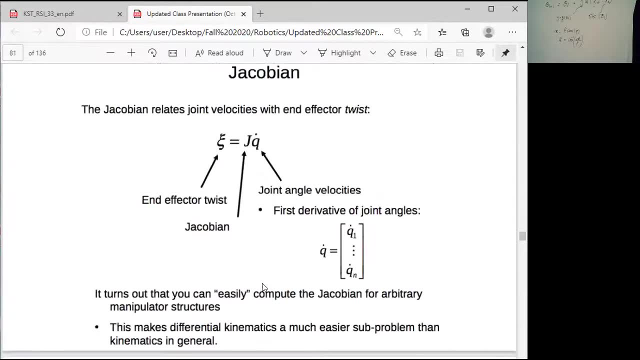 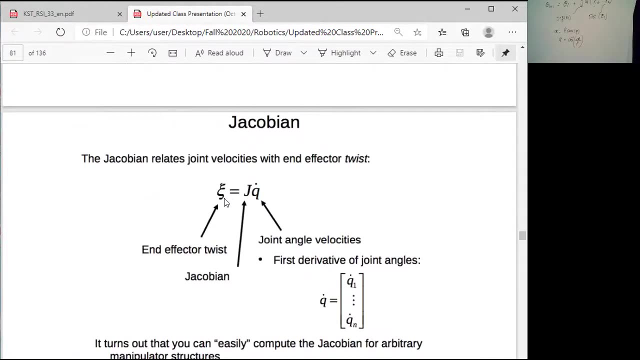 be able to do that, okay, guys. so, uh, if you apply this on a two degrees of freedom robot, if you have x, y, z again, you are also able to do that in a very nice and simple way: um and um, yep. so if you differentiate by dt, as i did earlier,